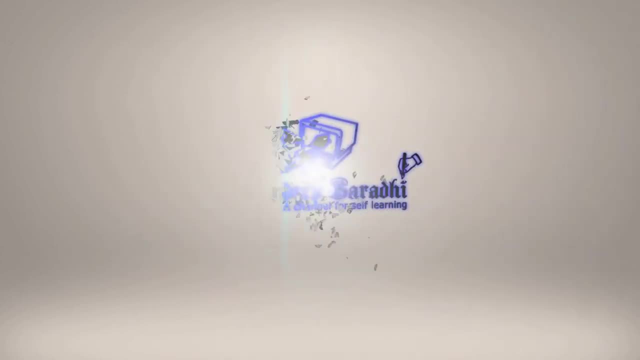 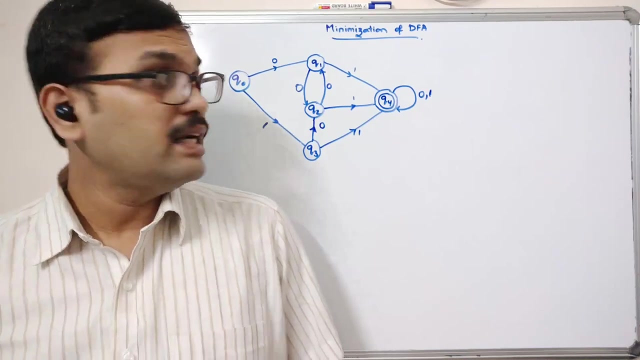 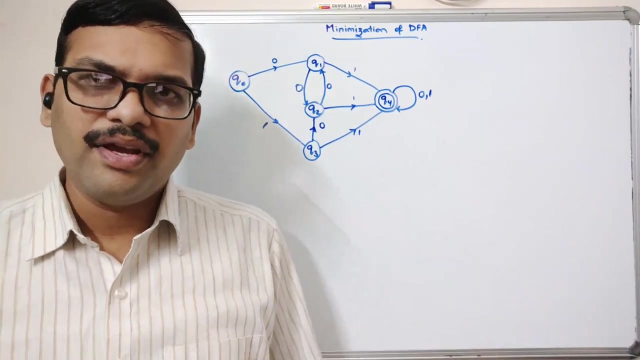 Hello friends, welcome back to our channel. So in today's session we'll discuss about one more topic in automata theory, that is, the minimization of DFA. So so far we have discussed about how to construct the DFA and how to construct the NFA, and also we have seen the conversion of NFA to 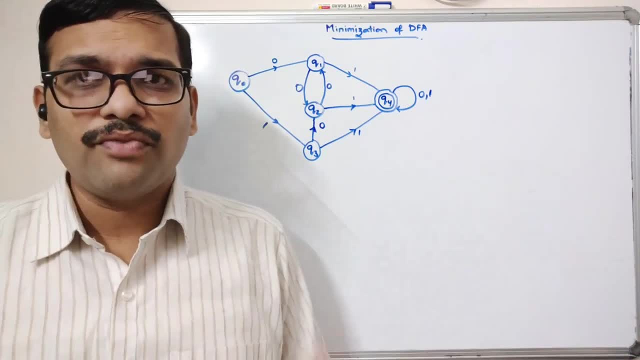 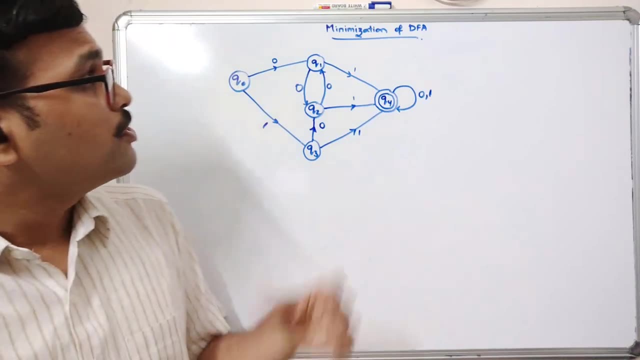 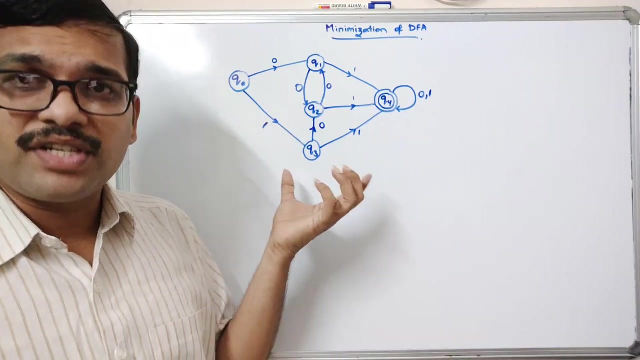 DFA, because the implementation is not feasible for NFA, so that we have to convert it to a DFA and the implementation can be done for the DFA. And now in this topic, so we'll see the minimization of DFA. So this is a complete DFA, but so is it possible to reduce the number of. 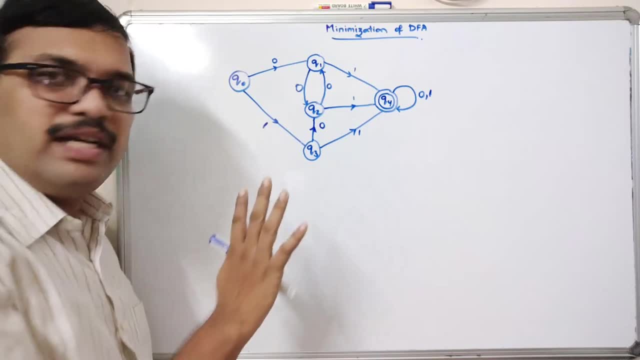 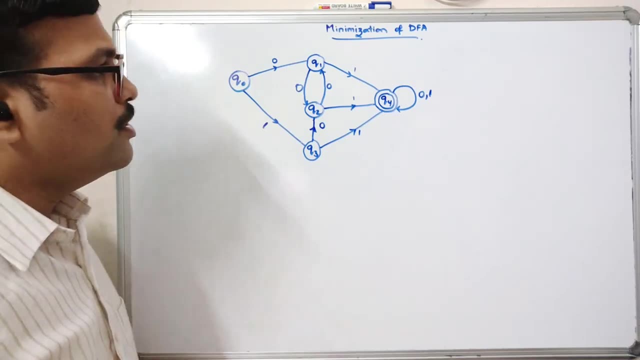 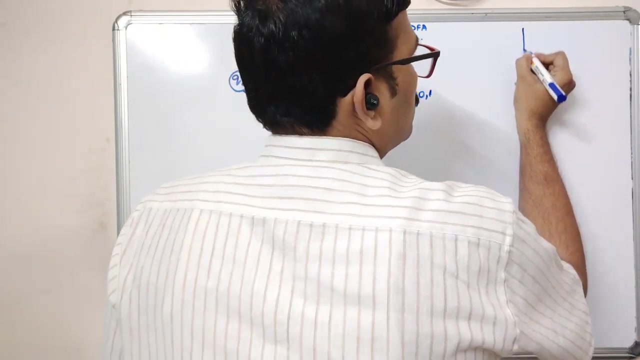 states. So here you can see in this example we are having around five states and is it possible to reduce the states? that means minimization of DFA, right. So first of all we'll take this example and we'll draw the transition table for this one. So the input symbols are two, zero and 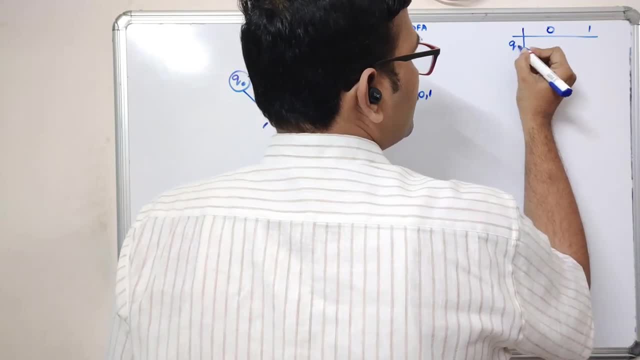 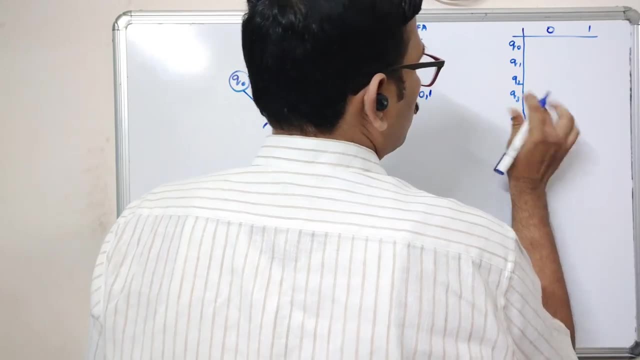 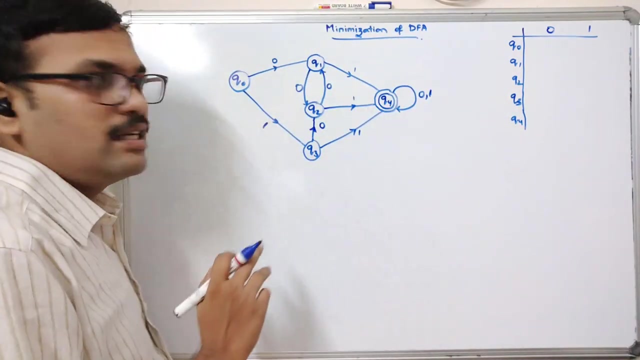 one. So for zero and for one, and the states are Q, naught Q1, Q2, Q3 and Q4.. So total five states. are there right? So these are the five states. Now we have to fill the transition table, So Q. 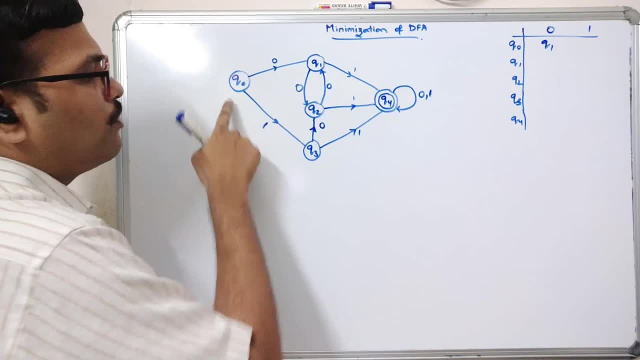 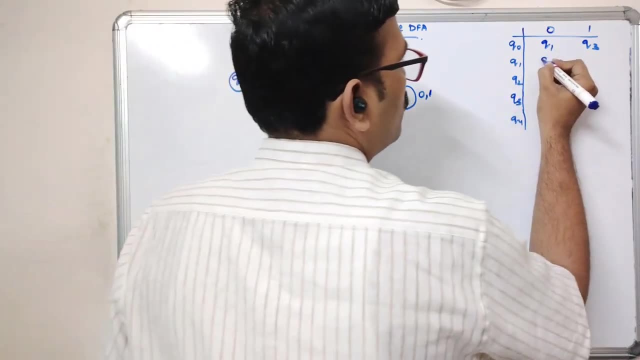 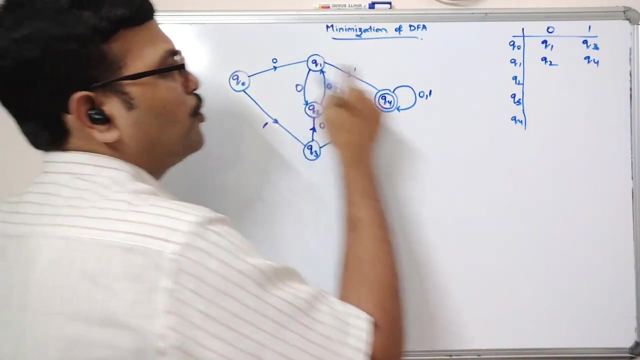 naught on zero, Q1.. We move to Q1 state And Q naught on one. it moves to Q3.. And Q1 on zero, it moves to Q2.. Q1 on one, it moves to Q4.. Q2 on zero: it moves to Q1.. Q2 on one, it moves to Q4.. 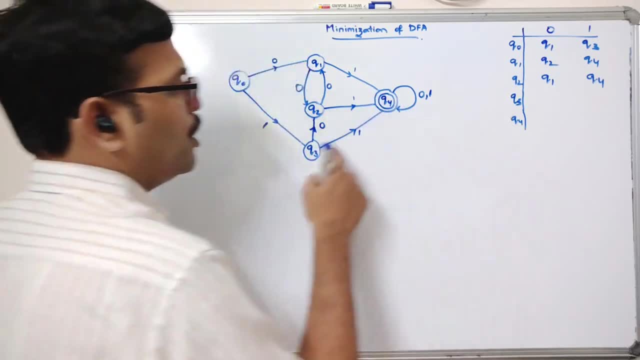 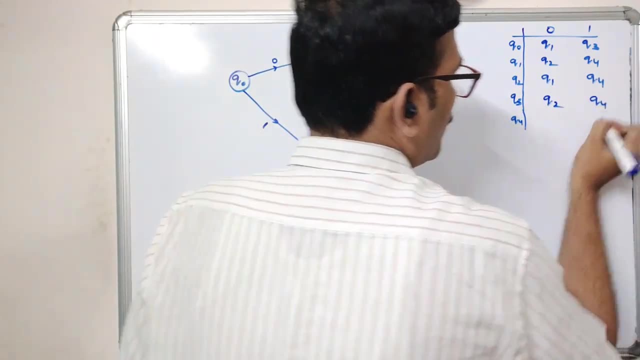 Q3 on one, It moves, sorry. Q3 on zero, it moves to Q2,. Q3 on zero, it moves to Q2.. Cool Now. 3 on 1, it moves to Q4.. Q4 on 0 and 1, the self-transition: it remains in the same state. 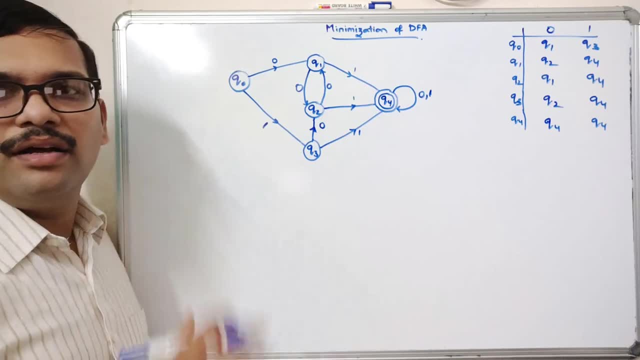 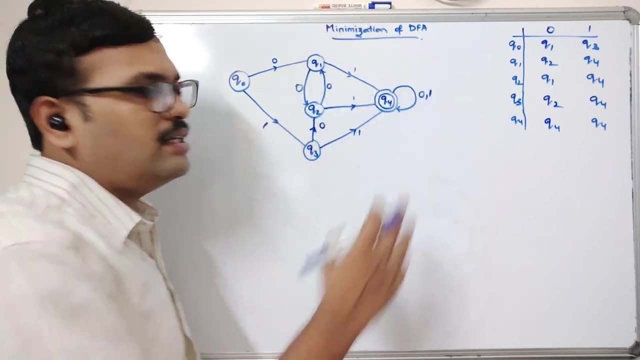 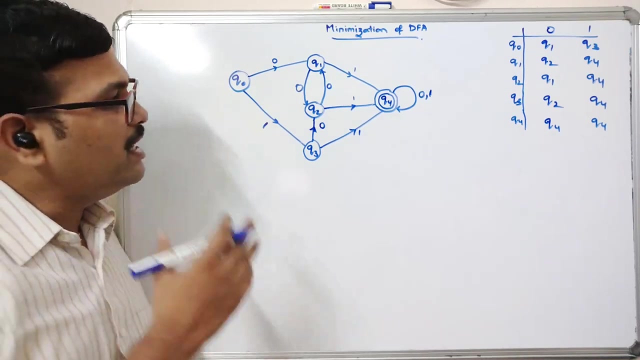 So this is the transition table for the given diagram. Now the next step is we need to divide the complete states into two sets, That is, one with the non-final states and another with the final states. So we know that the DFA can have a multiple final states. But here, in this example, 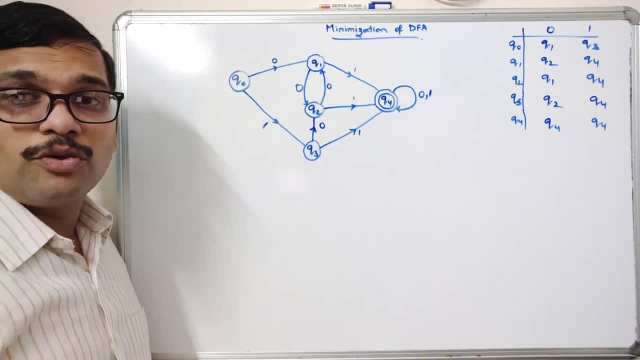 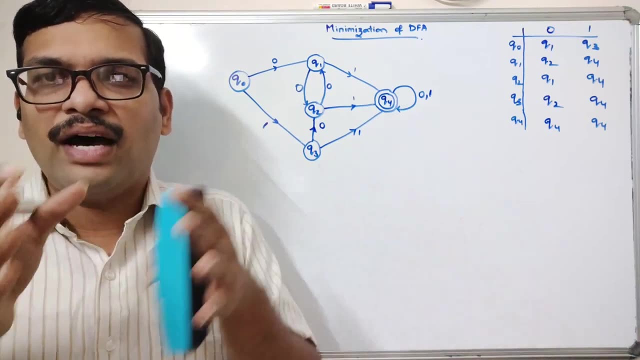 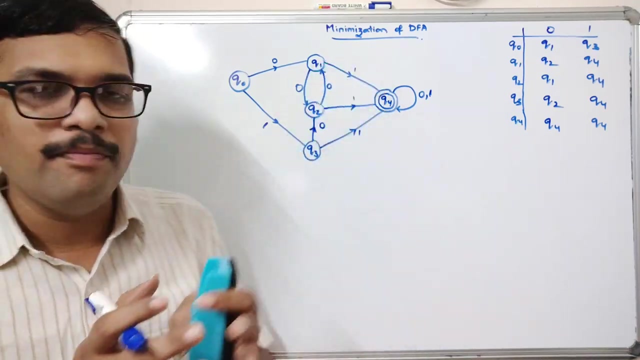 we are having only one final state, So. but the first step is we need to find the two different sets: one set with the non-final states and another set with the final states, So that we call it as a zero equivalence. So in this minimization problem, so we need to find the 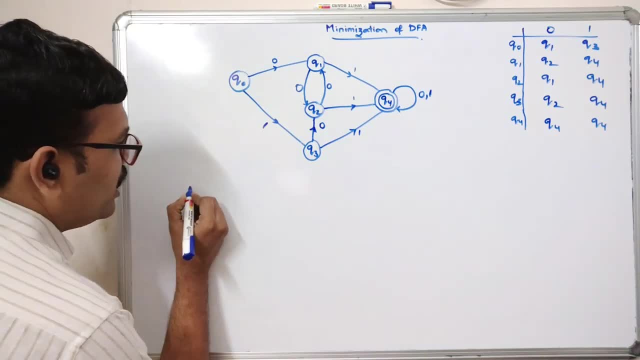 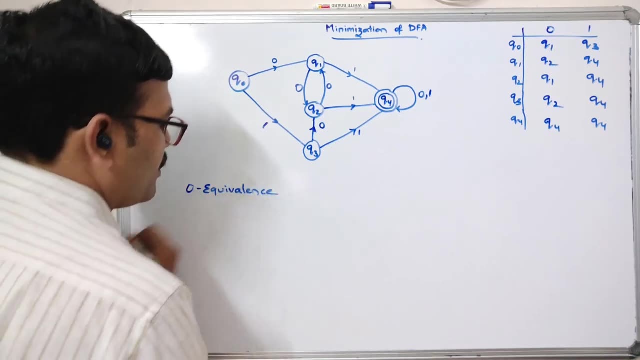 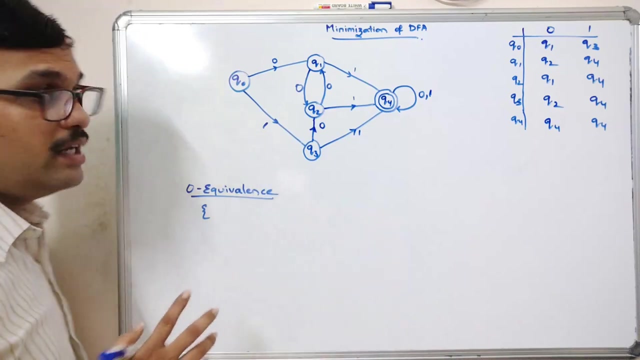 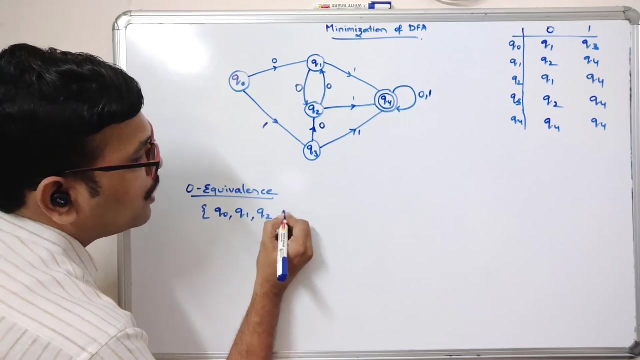 equivalence. So first one is zero equivalence. So here we are having two sets, one with the non-final sets and another one with the final states. So here non-final states are Q0, Q1, Q2 and Q3.. So from this diagram you can see all. 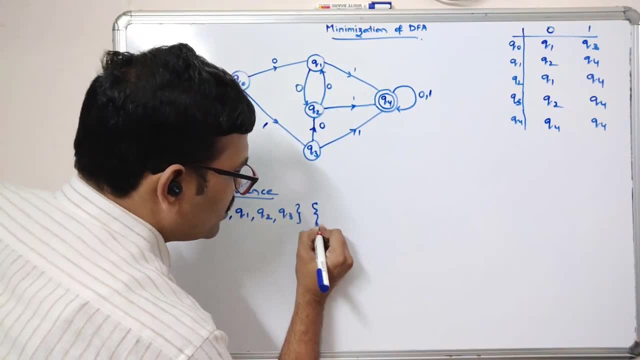 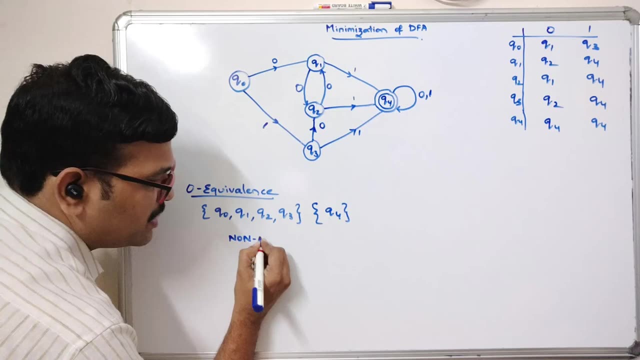 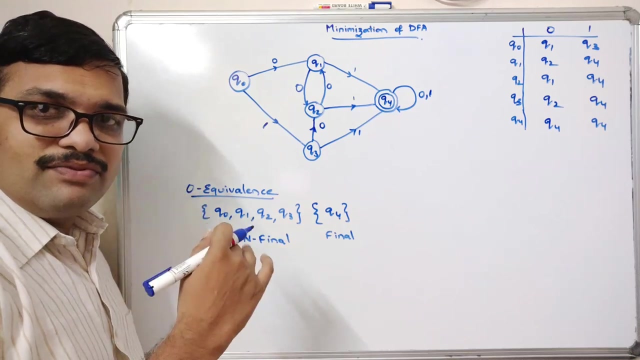 these four are the non-final states, And there is a one more state called Q4, which is a final state. Non-final states, okay, non-final states and final state. The first step is this one, okay, And from this one we need to find the one equivalence That. 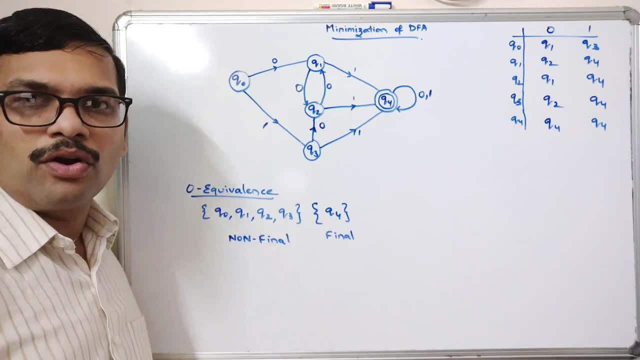 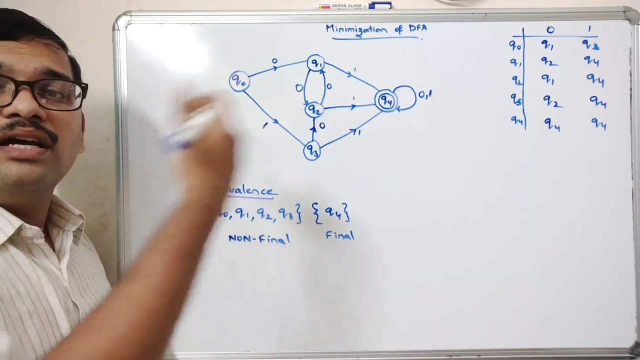 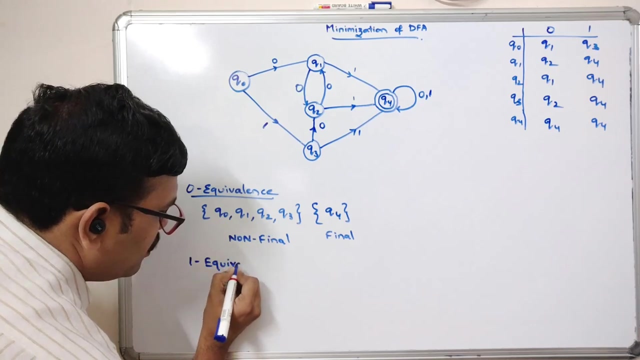 means we have to find whether these two states are equal or not. So that means equivalence of states you should be find and if they are equal it remains in the same set, Otherwise it fall in the new set. okay, So let us check with the one equivalence, See whenever you are finding the 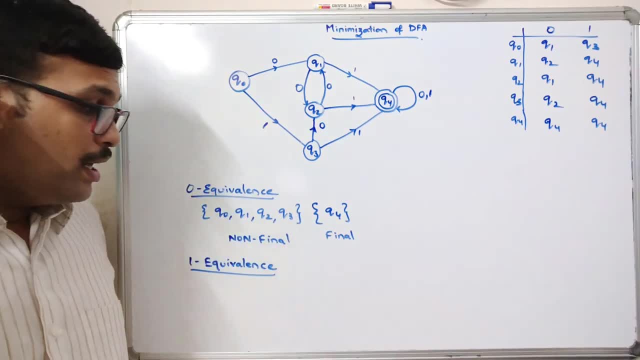 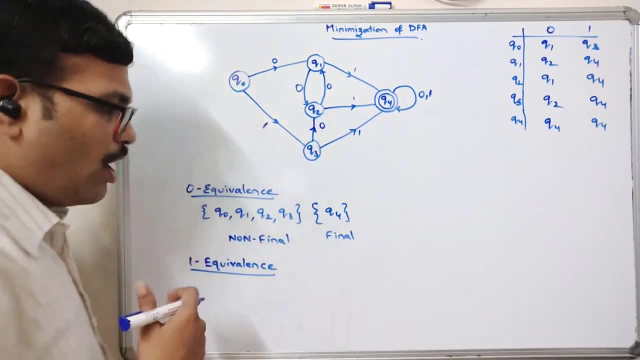 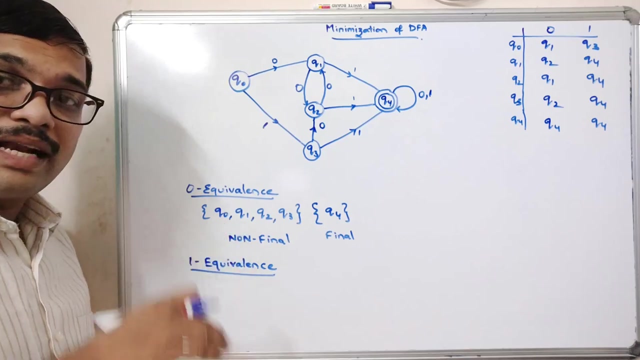 equivalence. we will have to compare the two states. So let us check with the one equivalence. Now we have to compare Q0 with all the remaining states, whether it is equal or not. right, How can we compare this one? So, over the input symbol 0 and 1, compare the two states, the resultant: 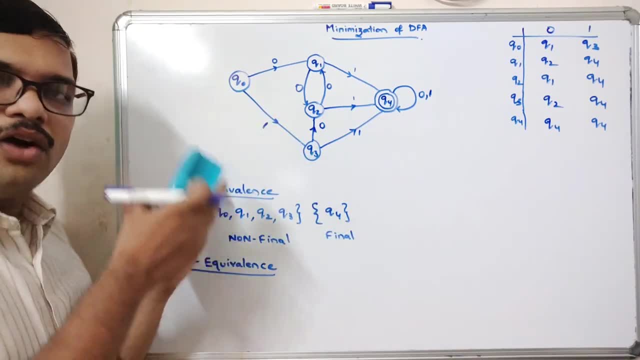 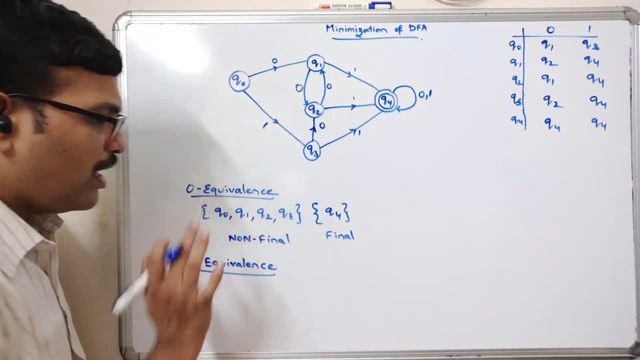 states. If the resultant states fall in the same set, then automatically it shows that two states are equal right. So let me explain you with an example. Now we will compare Q0 and Q1, okay, Q0 and Q1.. 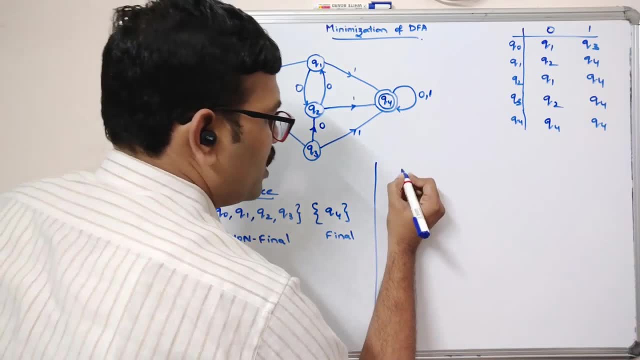 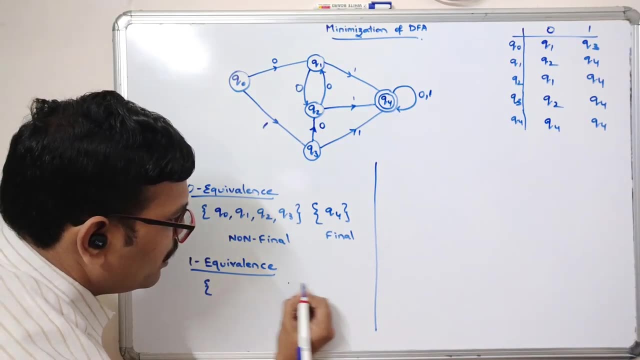 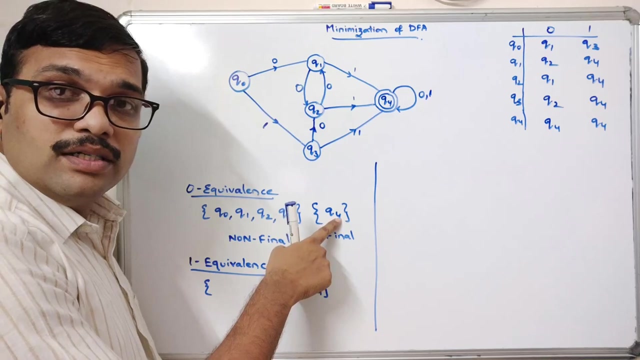 So I will explain here itself, okay, For the one equivalence. and see, here there is one set and automatically, here we are having one more set called Q4,. okay, Q4, because it is having only one state, So we need not compare with any other, So it will remain in the same state, okay, Now? 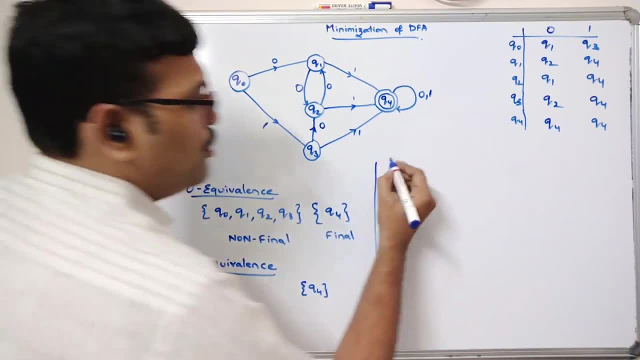 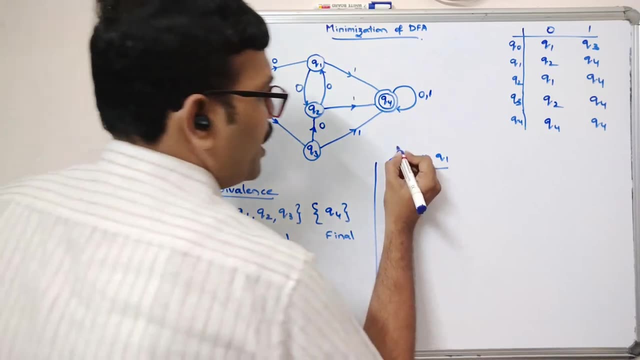 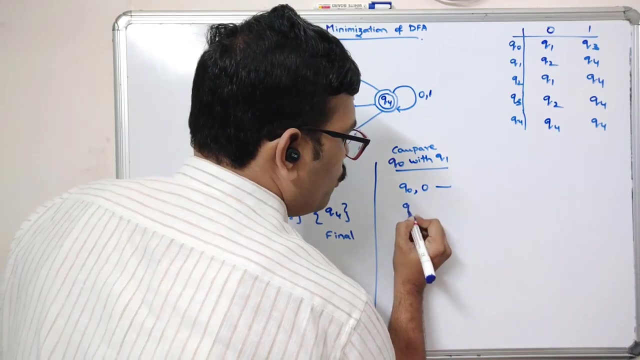 we have to compare Q0 with Q1, Q2, Q3.. Now we will compare Q0 with Q1, Q0 with Q1.. So compare, So we know that Q0 on 0 and Q1 on 0. Similarly, Q0 on- sorry, Q0 on. 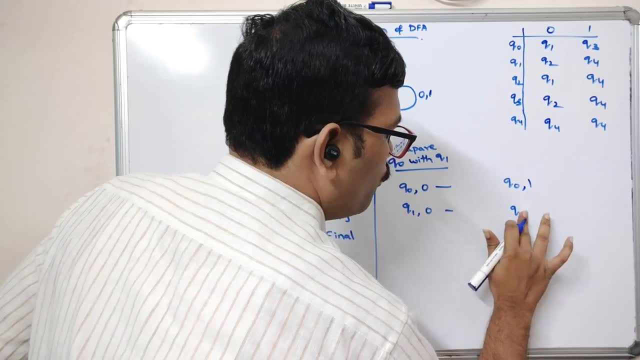 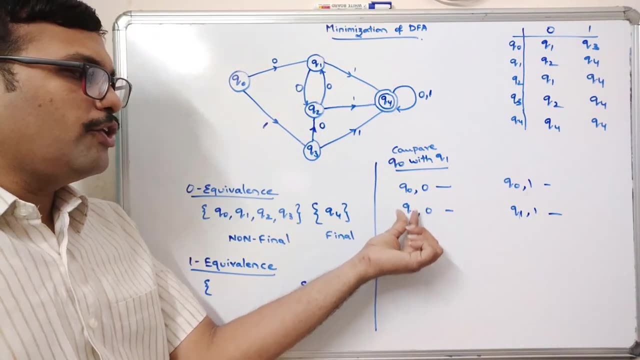 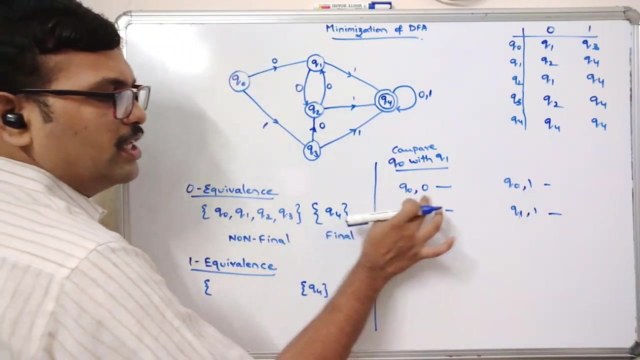 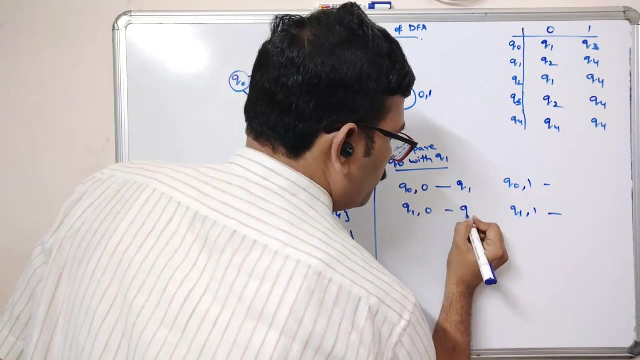 1 and Q0, sorry, Q1 on 1, Q1 on 1,. okay, So we are comparing the Q0 and Q1 over the input symbol 1.. Now we can observe Q0 on 0.. Q0 on 0,- it moves to Q1.. Q1 on 0,, it moves to Q2.. Just compare the. 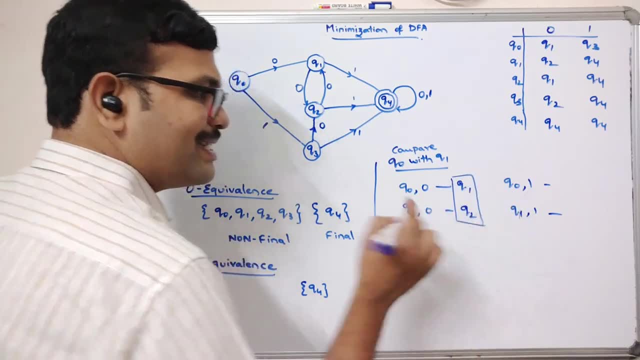 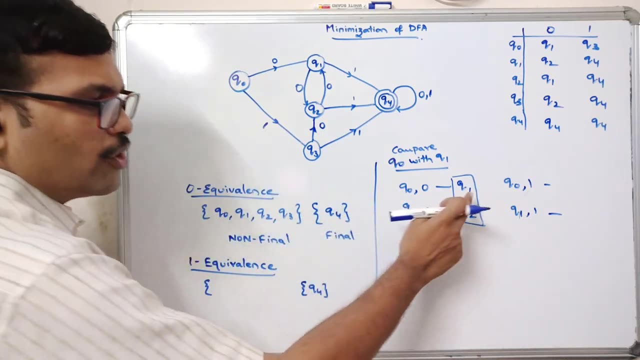 resultant states whether these states fall in the same set of previous equivalence. Here we are finding the one equivalence where we have to check in the zero equivalence You can see Q1 and Q2.. So fall in the same set. okay, Q1 and Q2 fall in the same set, So you can see Q1 and Q2 fall in the. 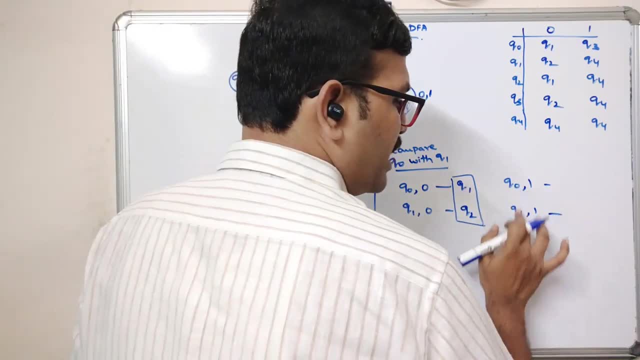 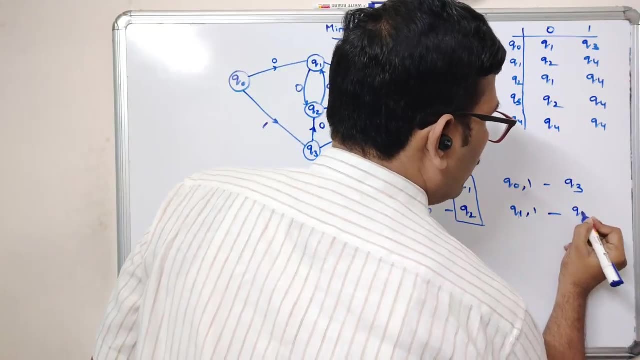 same set. right Now. compare this one: the states with input symbol 1.. Q0 on 1, it is a Q3, and Q1 on 1, it is a Q4. And here you can observe if these two states fall in the same. 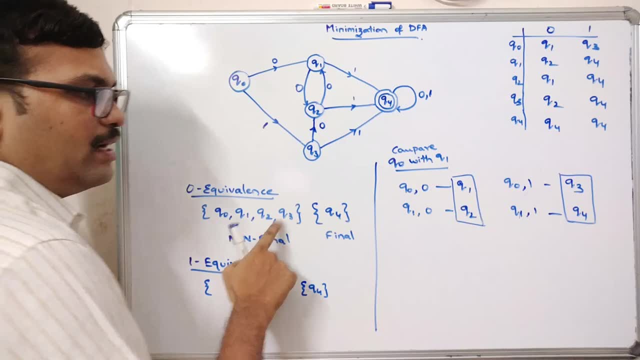 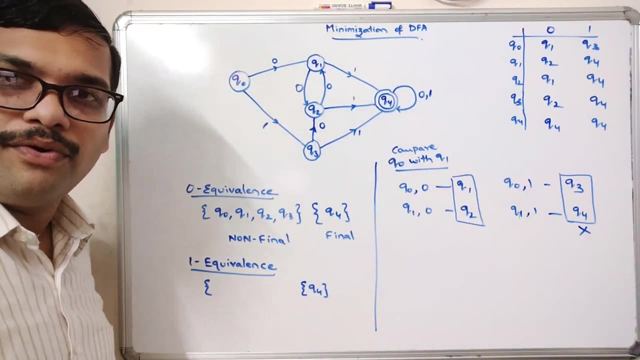 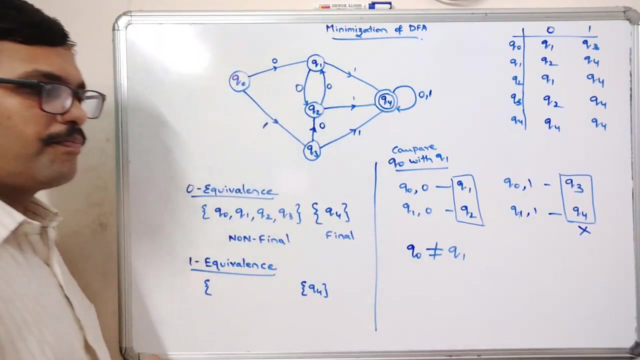 set or not. So Q3 is in one state, one set, and Q4 is in another set. So this implies: so this is not possible. okay, This is not possible. So that implies Q0 is not equal to Q1.. Q0 is not equal to Q1.. So that is why Q0 will be here and there will be one more set. 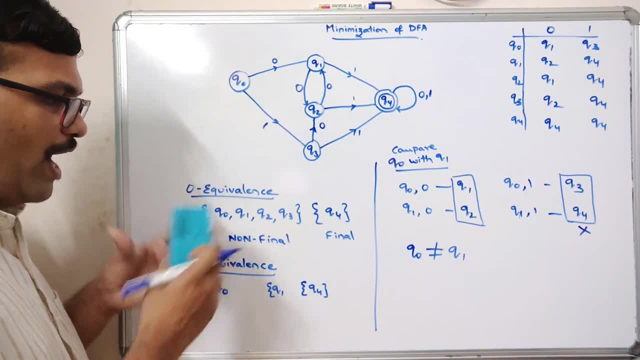 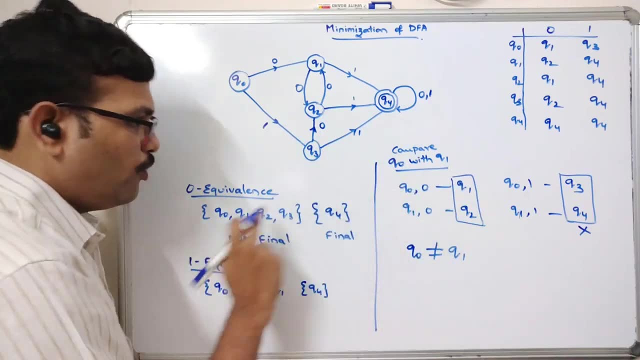 created and Q0 will be. remains here itself. okay, So we have to divide the unequivalent state to a new set, So Q0 and Q1,. if you compare Q0 and Q1, both are not equivalent, So we have to divide. 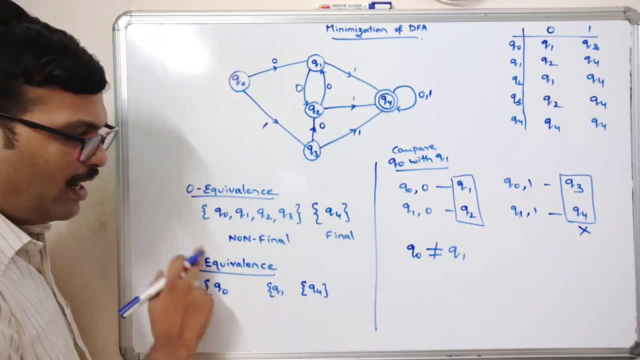 this Q0 and Q1.. So open the new set and just move the state which is not equal to Q0 to in the other. And now the next step: compare Q0 with Q2.. Same procedure. Now we need to compare Q0. 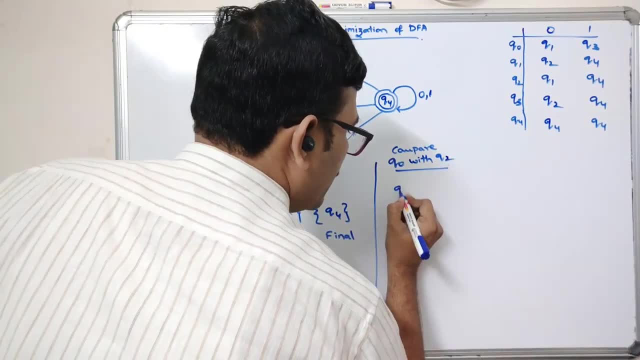 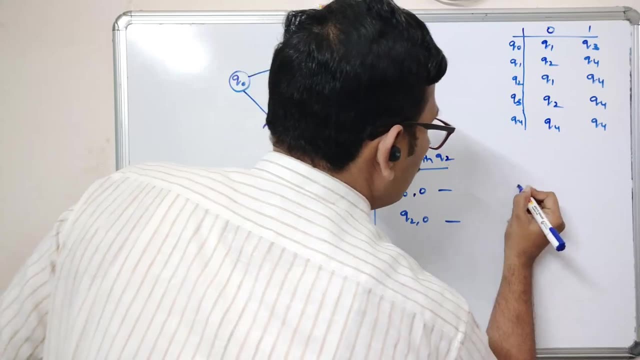 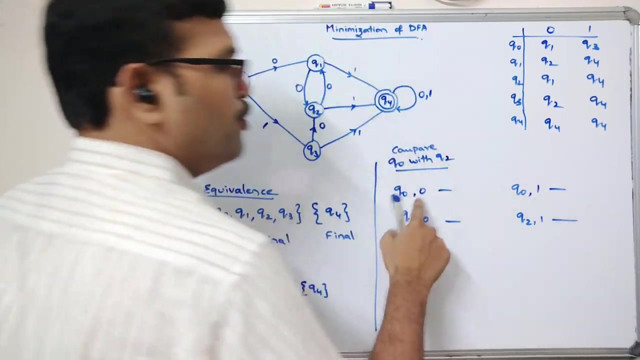 with Q2, Q2, right, Say Q0 on 0,. okay, Q0 on 0 and Q2 on 0. Similarly, Q0 on 1, Q0 on 1 and Q2 on 1.. Say Q0 on 0,, Q0 on 0,- it is a Q1 and Q2 on 0,- it is a Q2 on 0. So. 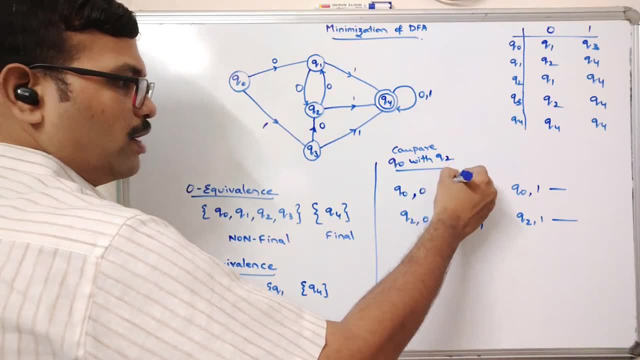 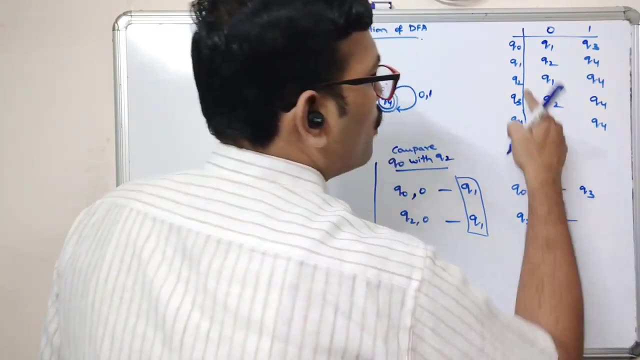 you can compare. So Q1, both are falling in the same set, Q1, right Next, Q0 on 1, it is a Q3, and Q2 on 1, it is a Q4. So again you can observe here, both are different, Both are different. Q3. 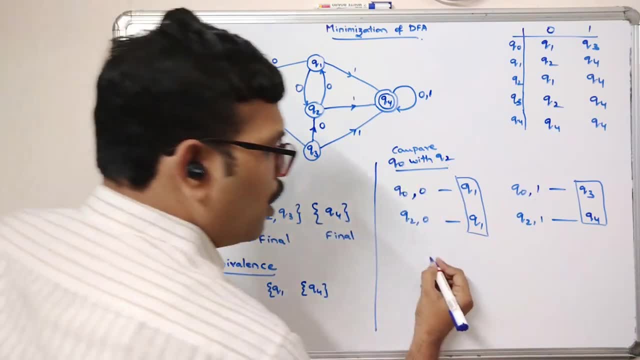 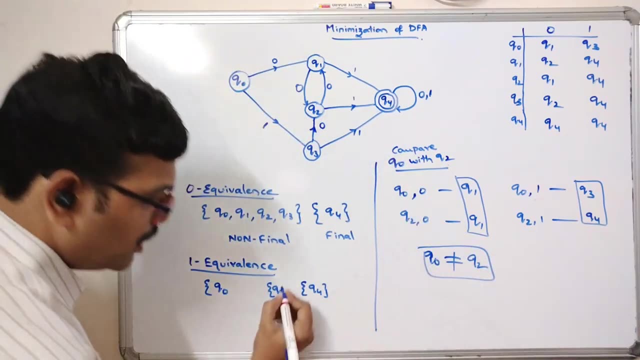 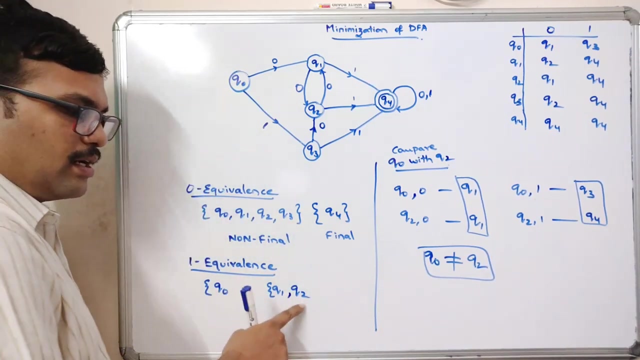 in one set and Q4 is in another set. So Q0 is not equal to Q2.. Q0 is not equal to Q2.. So we have to divide the Q2 also. So just insert the Q2 in the new set, okay. And now we need to compare Q0 with the Q3, because we have 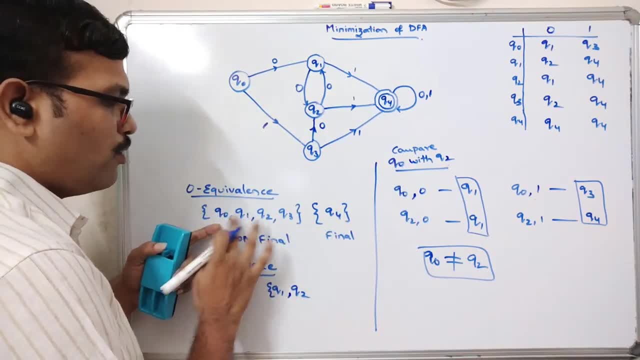 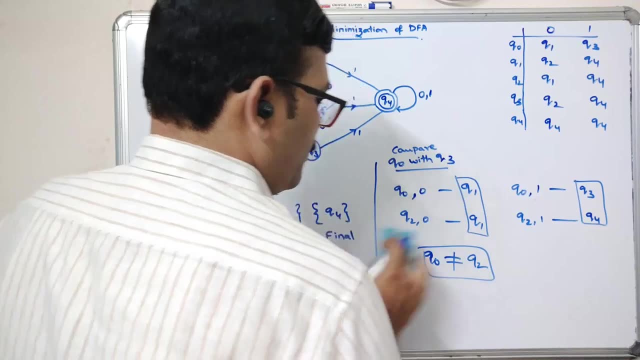 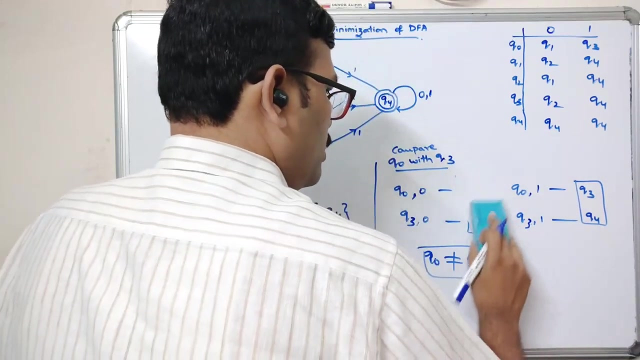 compared Q0 with Q1, Q0 with Q2.. Now we have to compare Q0 with Q3.. Now see Q3, and here also we need to find Q3 on 0 and Q3 on 1.. Now so let us repeat the same process. 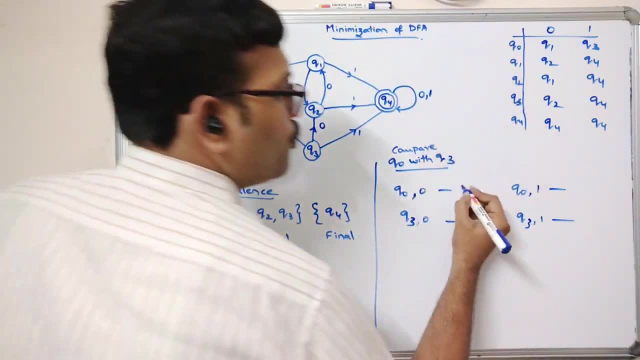 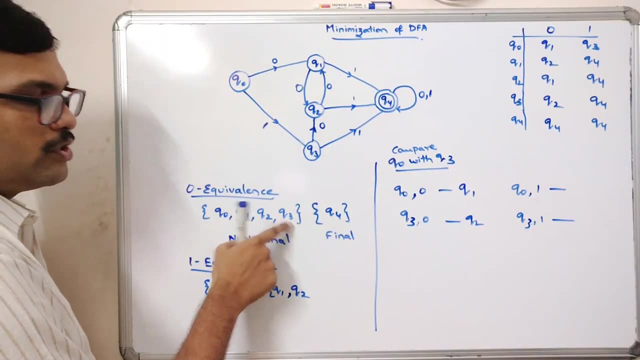 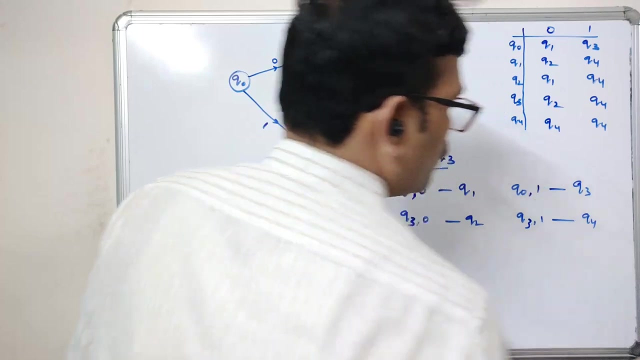 So Q0 on 0, it is a Q1 and Q0 on 0, it is a Q2.. Both are in the same set: Q0, Q3, sorry, Q1 and Q2, right. Q0 on 1, it is a Q3.. Q3 on 1, it is a Q4.. It is a Q4.. Again, this is not equal, So again. 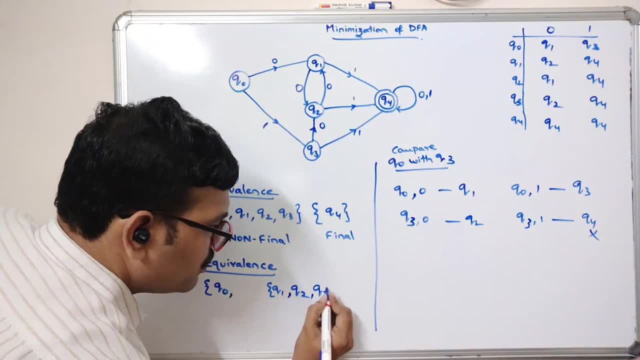 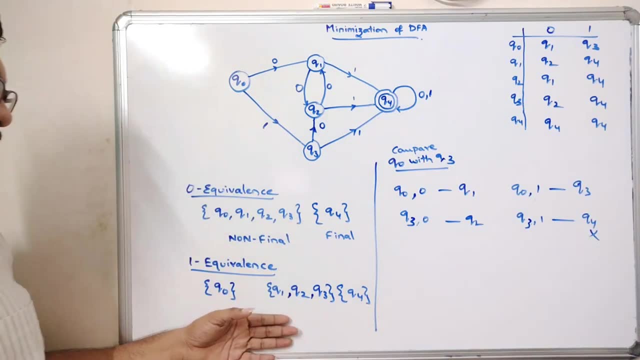 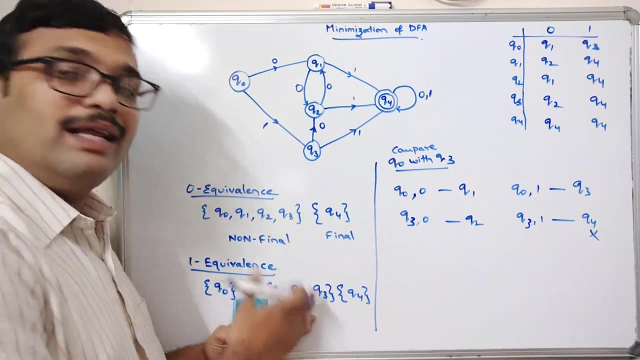 we need to divide Q0 with a Q3. So Q3 falls in the new set and Q2 will. Q0 will be remaining in the same set. So this is the one equivalence. So after one equivalence, the Q0 is in one set. Q1,, Q2, Q3 are in another. 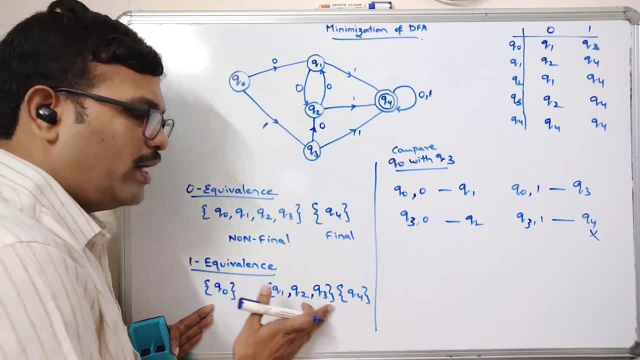 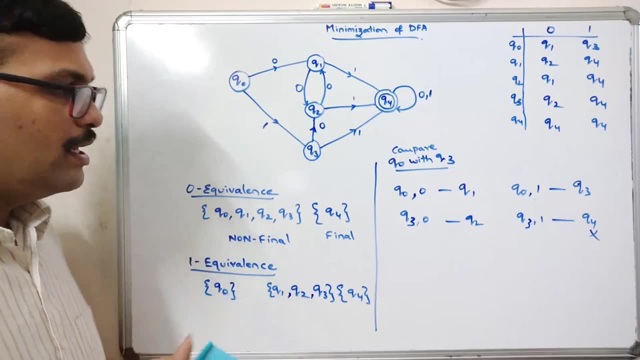 set, because Q0 is not equivalent to Q1, Q2 and Q3. So that is why we are dividing the set, So we are reducing the states of a set. okay Now, so this is the procedure to form. 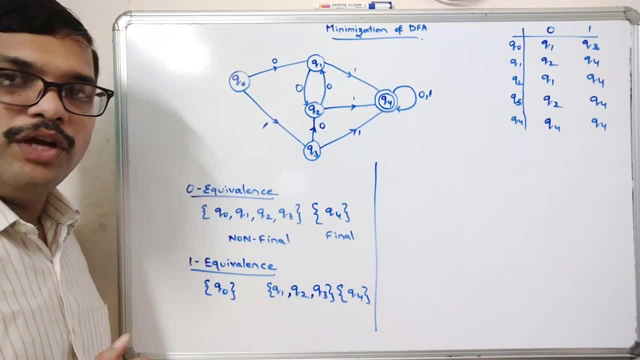 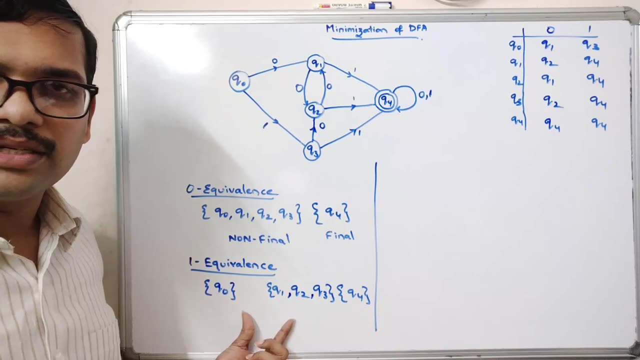 to find out the one equivalence. After that we need to find the two equivalents And then three equivalents. So we need to repeat the same process until we get the same result in the consecutive equivalences. Now let us take with the two equivalents. Okay, 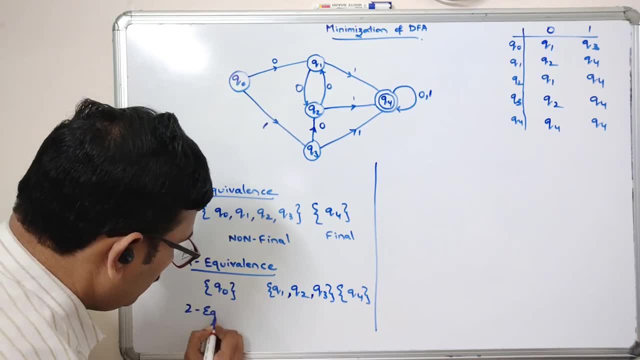 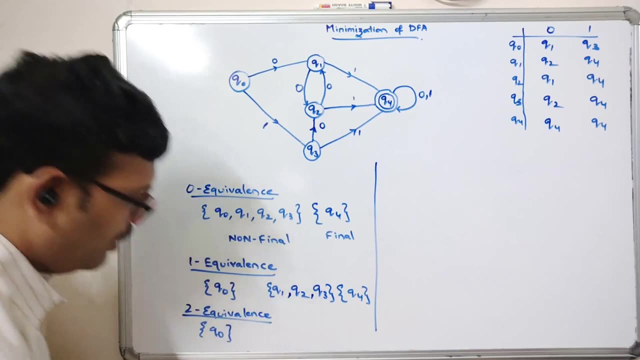 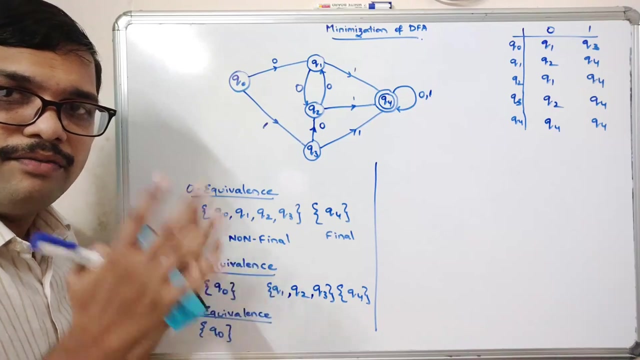 I will write here itself. I will write here itself. So two equivalents, right? So here you can observe: Q0 is a single state, So you need not change it, And we need to compare the Q1 with Q2 and Q3. And we have to divide that with an equivalence and non-equivalence. Now 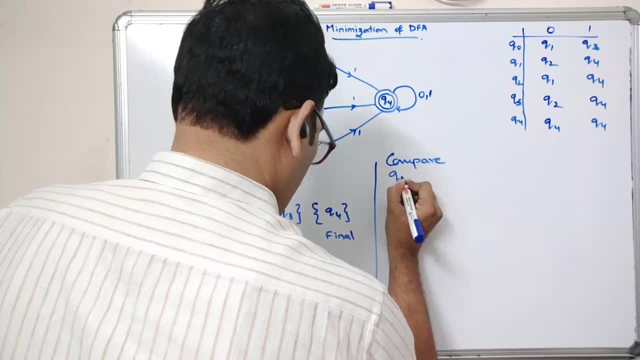 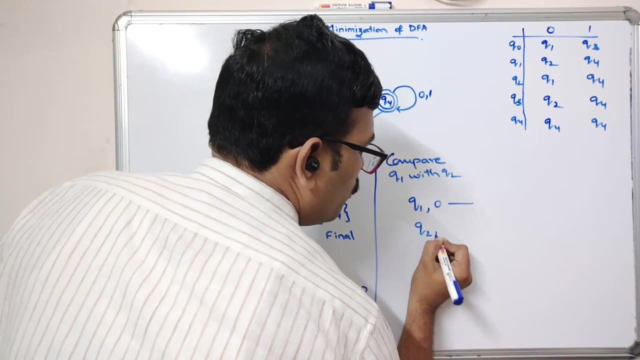 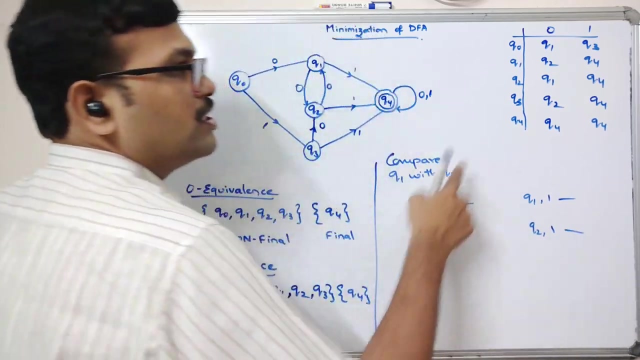 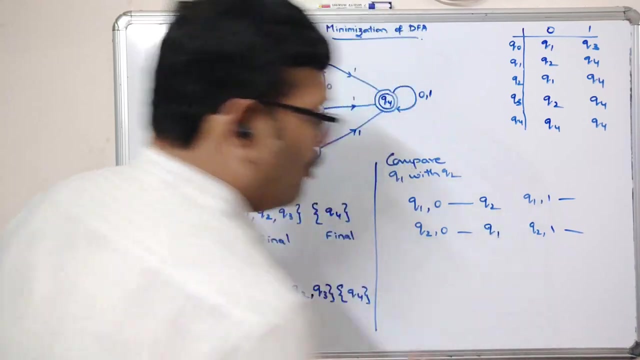 just compare Q1 with Q2.. So Q1 on 0, Q2 on 0.. Similarly, Q1 on 1, Q2 on 1.. So Q1 on 0, Q1 on 0. It is a Q2.. Q2 on 0. It is a Q1.. Now you have to check this one with the previous equivalent. So. 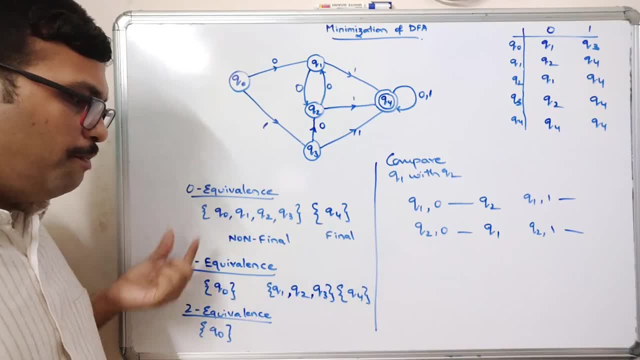 we are finding the two equivalents, So we are finding the two equivalents. So we are finding the two equivalents. We have to compare it with the one equivalents. So before we have, we are finding the one equivalent. So we have to compare the zero equivalents. Now you can see Q2. 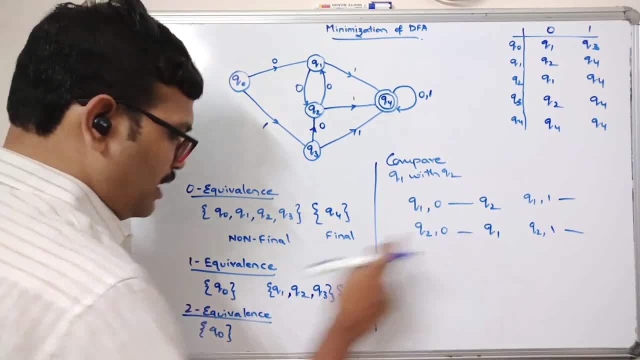 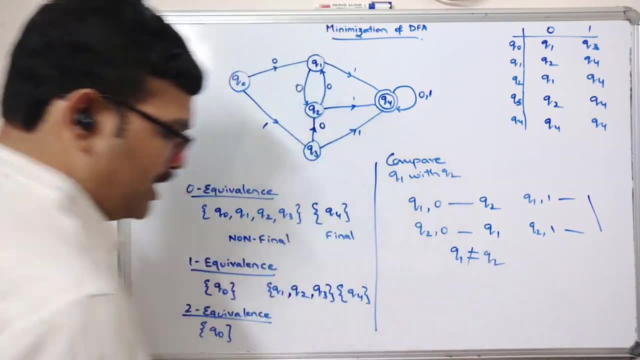 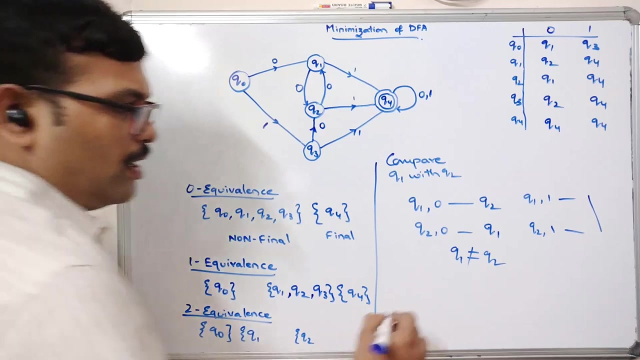 and Q1.. So Q2 is in one set and Q1 is in another set, So you need not find out this one. So Q1 is not equal to Q2.. So just divide the Q1, Q2.. Okay, And now hope you understood Q1 and Q2.. 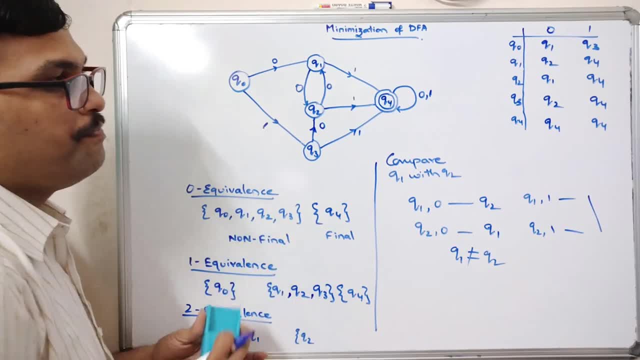 Now you just divide the two equivalents, So you need not change it. So you need not change it. So now you just find the. compare the Q1 with Q3.. Just compare the Q1 with Q3.. So you compare the. 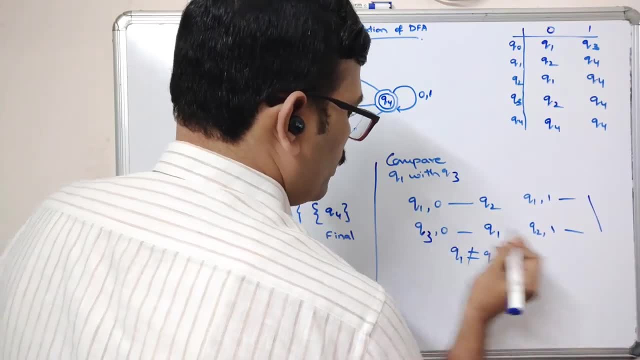 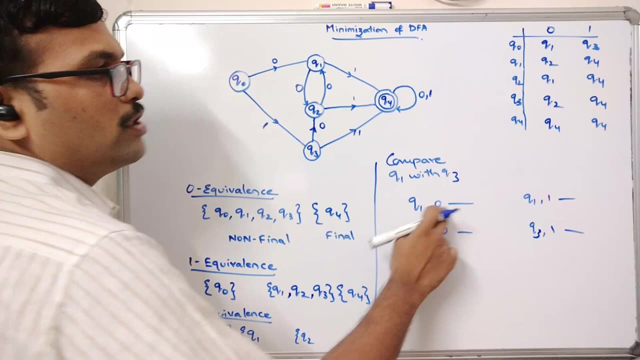 Q1 with Q3.. So here also I will go with the Q1 and Q3 and Q1 and Q3 and see now whether both the states are equal or not. So Q1 on 0 is a Q2.. Q3 on 0 is a Q2.. So you can find, you can find. 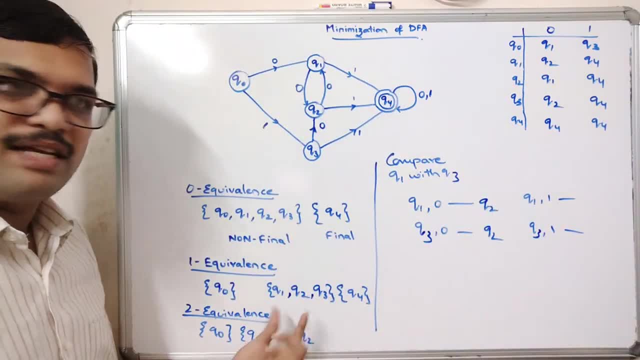 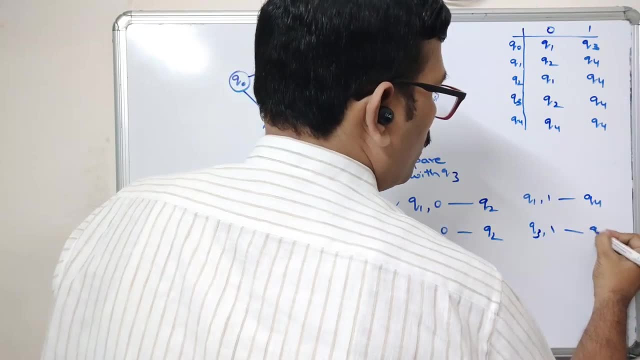 these two are the same state, which falls in the same set. So this is equal: Q1 on 1, it is a Q4.. Q3 on 1, it is a Q4.. So both are in the same set. Okay, Both are in the. 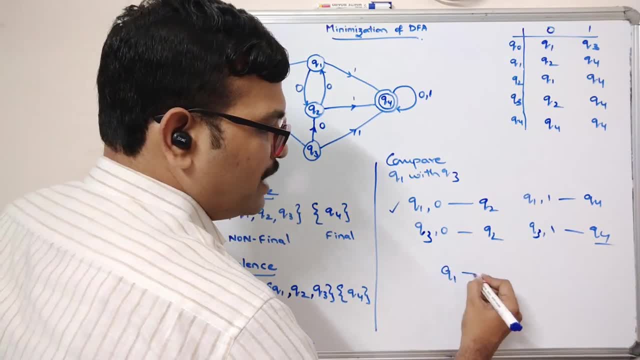 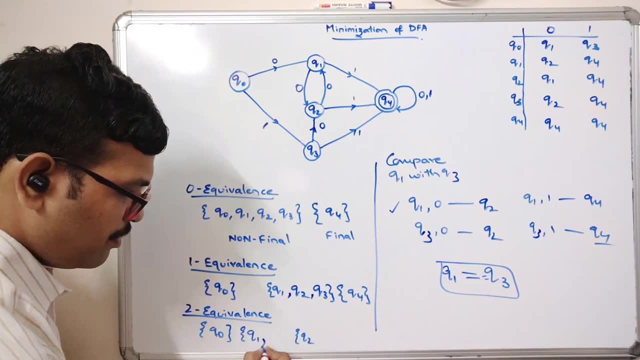 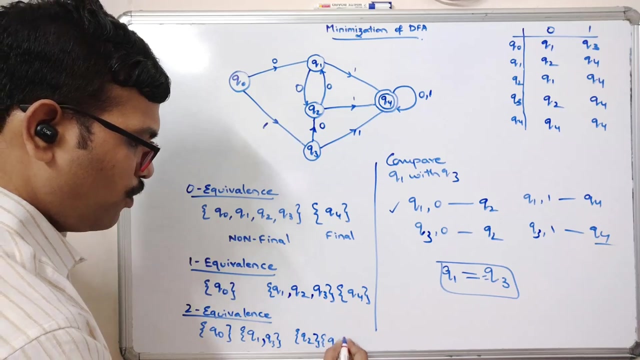 same set Q4.. Okay, So that implies: so Q1 is equal to Q3.. So both are equal. So just place it here: Q1 and Q3 and Q2, and again it is a Q4.. Now you can observe here the two equivalents. 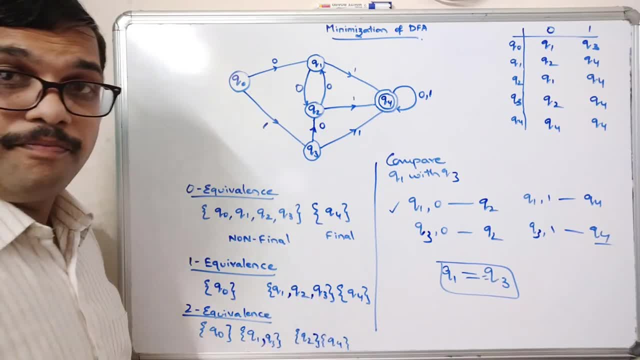 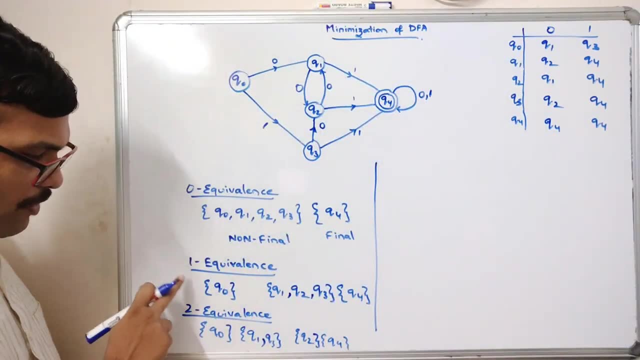 Q1, Q3 are same, Q2 and Q4.. Okay Now, now we need to find the three equivalents. We need to find the three equivalents because equivalents 1 and equivalents 2, both are not equal, Right, So? 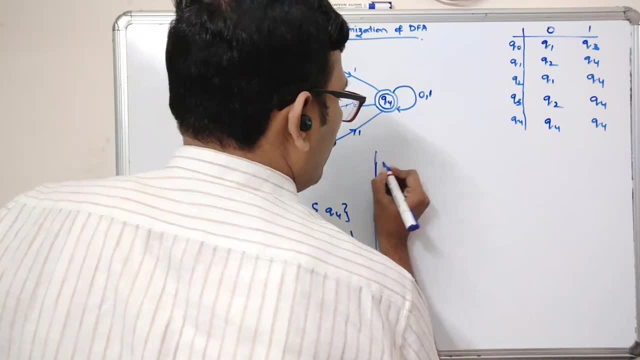 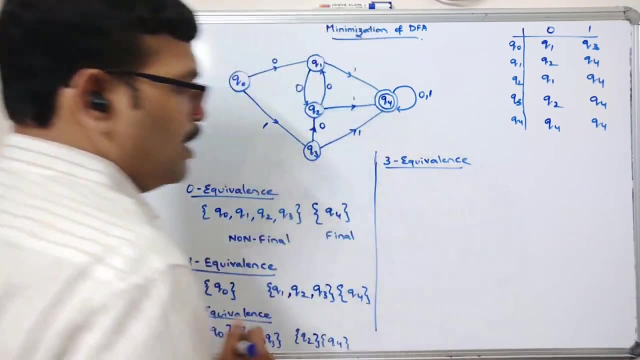 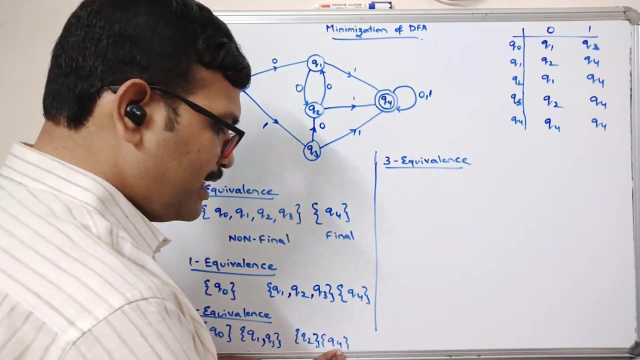 we need to find the equivalents 3.. So now just find the three equivalents. Three equivalents. So in the three equivalents we need to compare Q1 and Q3, because Q0 is a single state, Q2 is a single state and Q4 is a single state. So we are having the two states here. Now we need to. 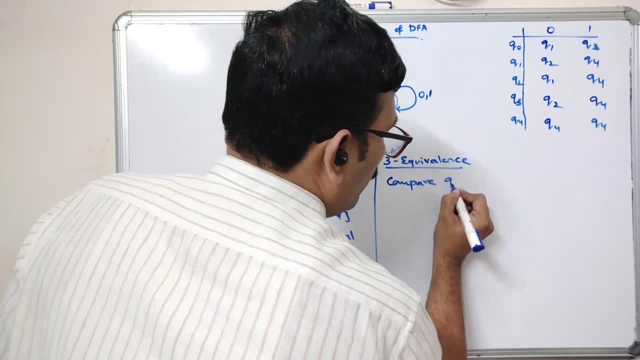 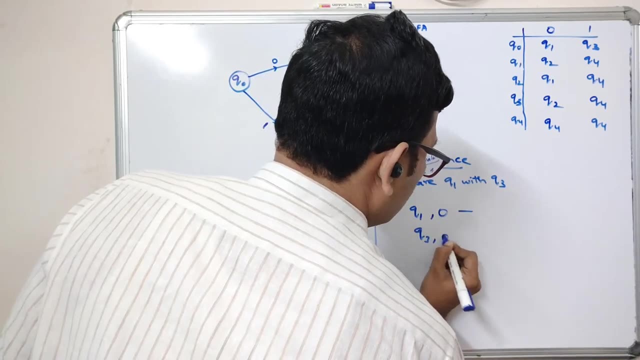 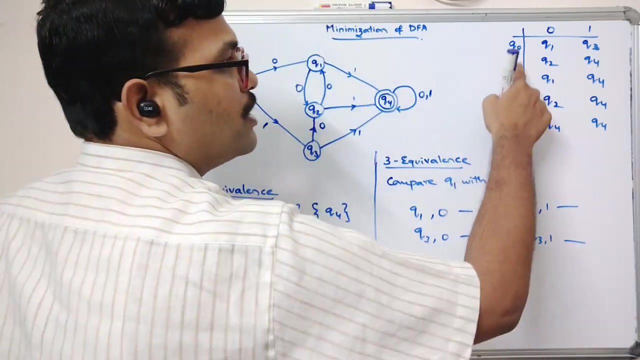 compare Q1 with Q3.. So Q1 on 0, Q3 on 0.. So Q1 on 1, Q3 on 1.. So you can see Q1 on 0, it is a Q2 and. 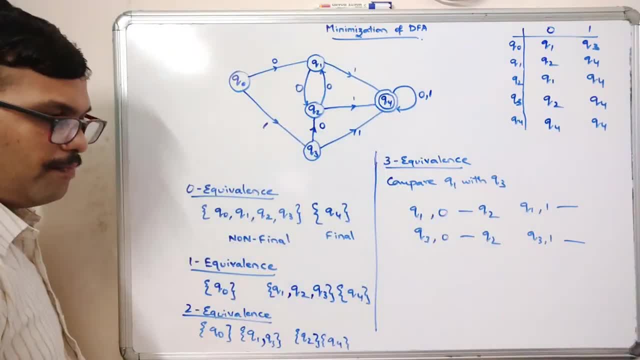 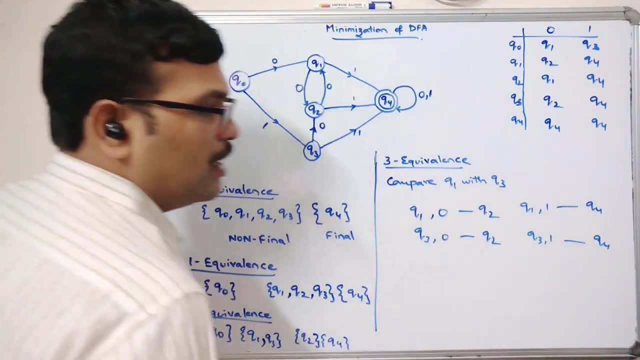 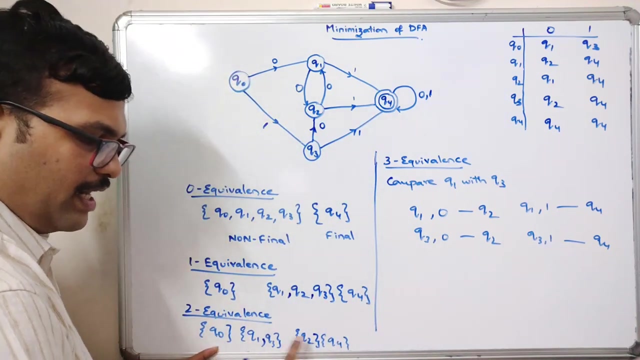 Q3 on 0, it is again Q2.. So both are equal Right, Coming to the Q1 on 1, Q3 on 0, Q3 on 1, Q3 on 1.. So simply, the third equivalents for this one is Q0, the single state. Q2- single state. Q4- single state. 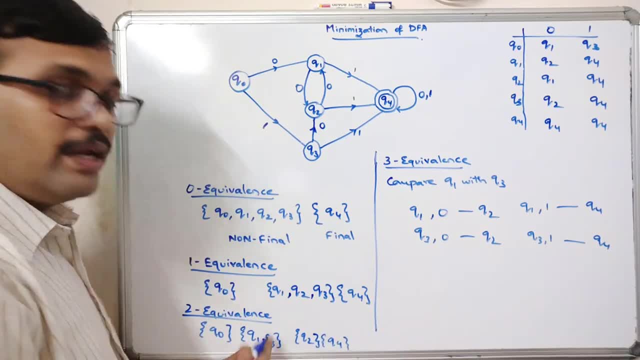 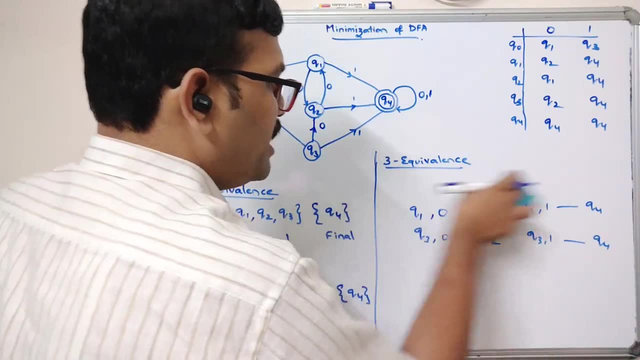 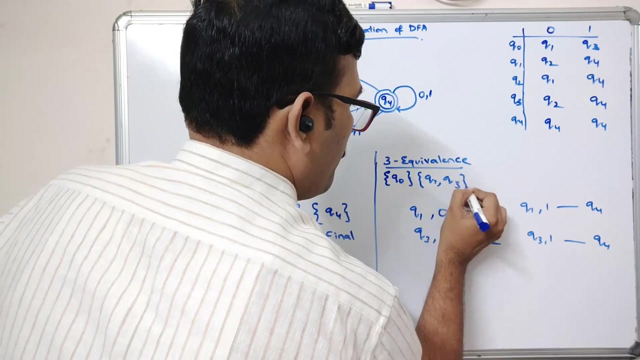 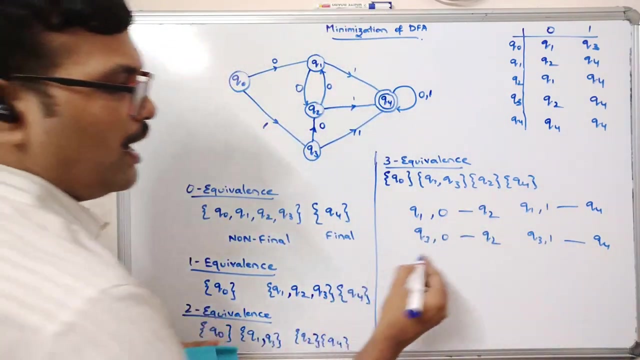 here we can observe three equivalents. the three equivalents is Q0, Q1 on 1, Q3 on 1, Q4 on 1, Q3 on Q1, Q3, Q2, Q4, because Q0, Q3 are equal. here Q1, Q3 are equal, so you can see the resultant. 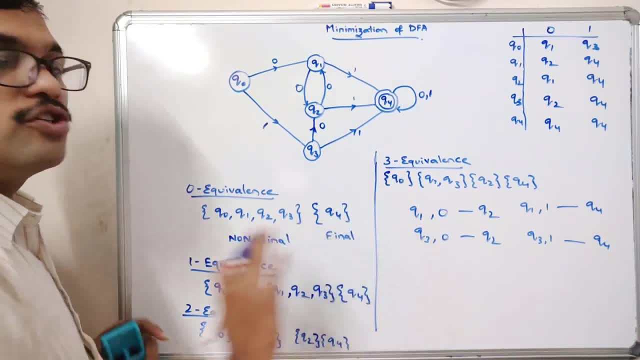 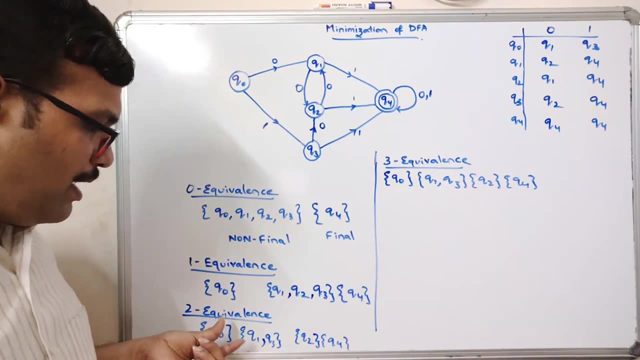 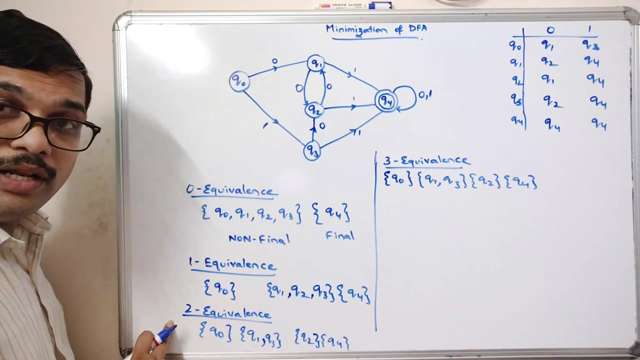 of third equivalence resultant of second equivalence. both are equal. so just stop finding the equivalences right. so we have to repeat the process until we get the last two equivalences result as same. so here one equivalence and two equivalence are. both are not equal, so we are finding the 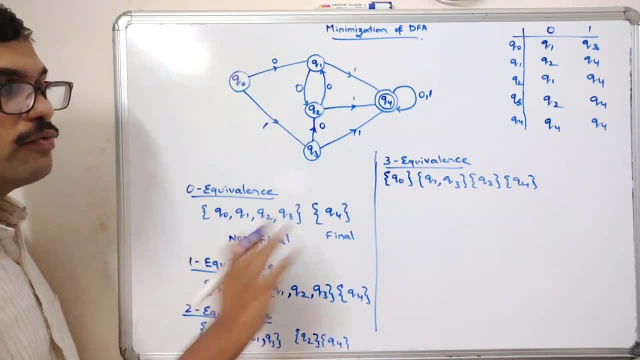 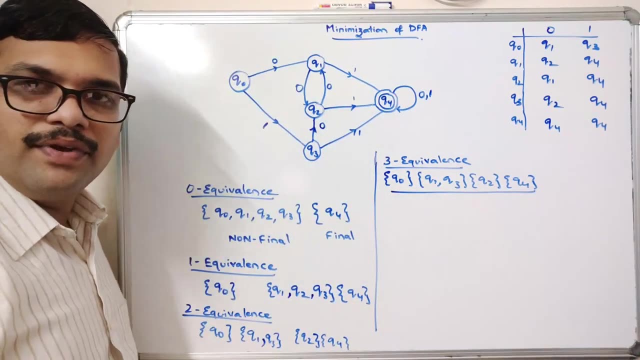 third equivalence. so third equivalence and second equivalence are equal. so we have to find out. I mean, we have to stop the procedure now by using this one. you have to draw the DFA. so here you can observe: Q0 is one state, Q1, Q3 is one state, Q2 is one state and Q4. 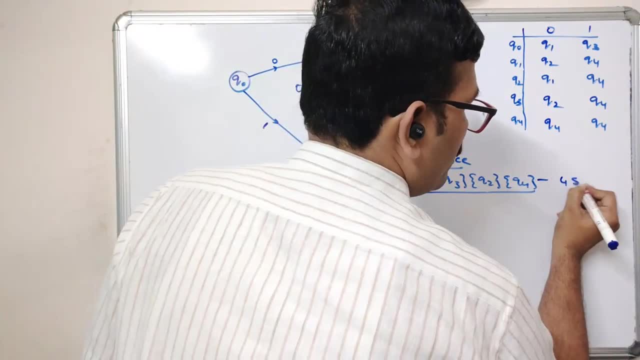 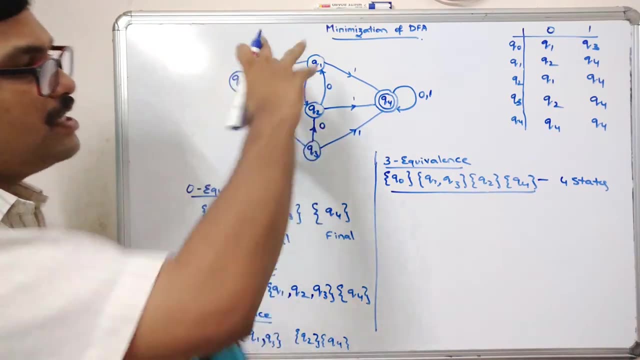 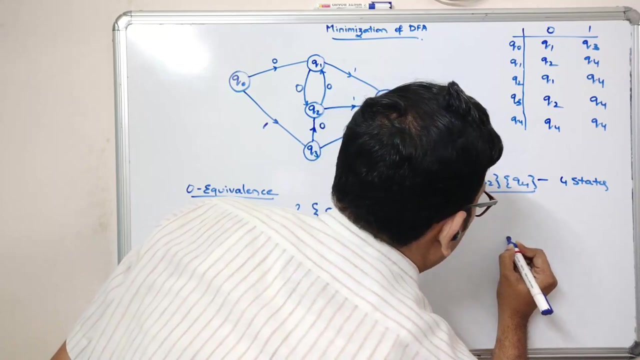 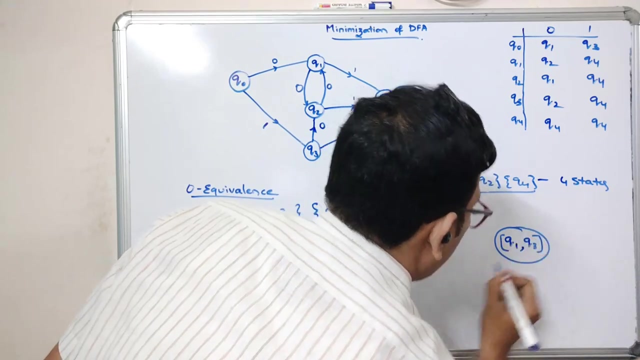 is one state, so total four states. so here you can say: the total states are four. but before minimization, how many states are there? there are five states, so here you can see states. so we are minimizing the five states to four states. so just find out, here the Q naught Q1 comma. Q3 becomes one state, Q2 is one state, Q4 is another. 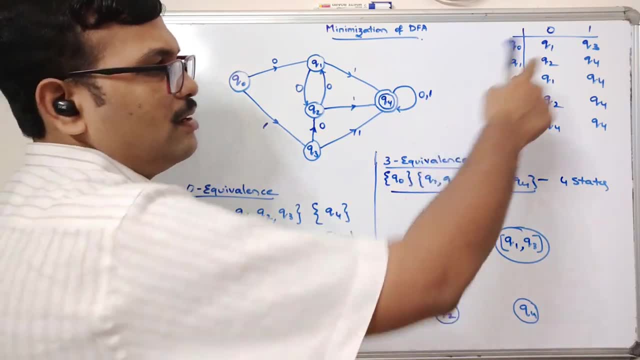 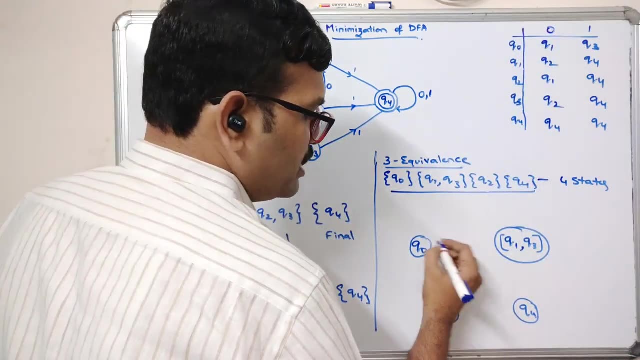 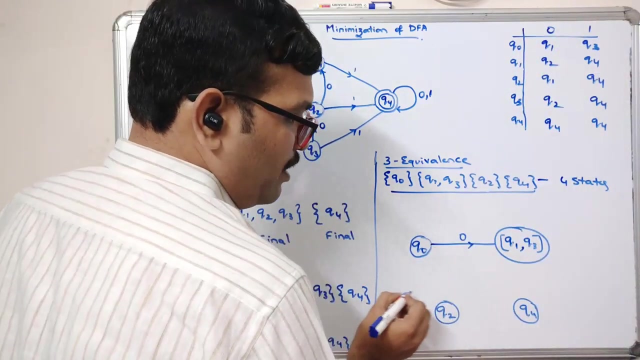 state: okay, four states. now just follow the transition table and find out the. I mean give the transitions Q0 on 0, Q1. so where is Q1?? Q1 on 0, it goes to Q1. Q0 on 1, it goes to Q3. so here itself. so 0 comma 1. 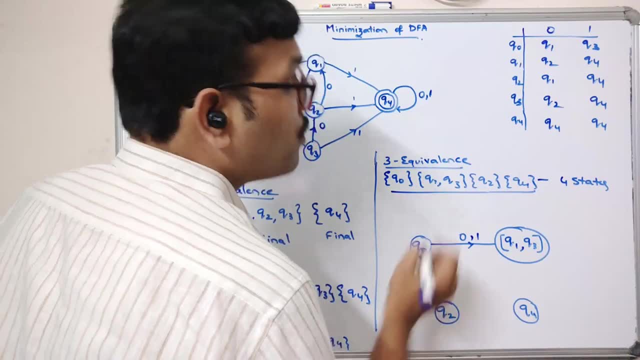 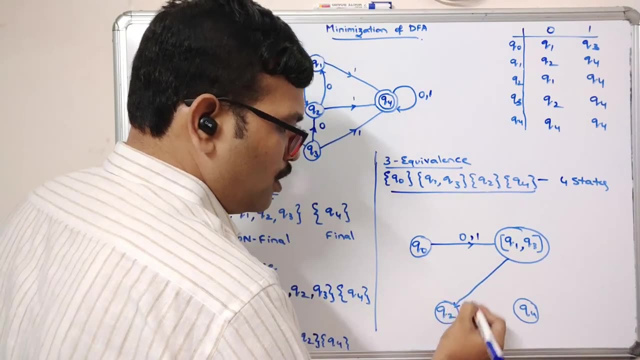 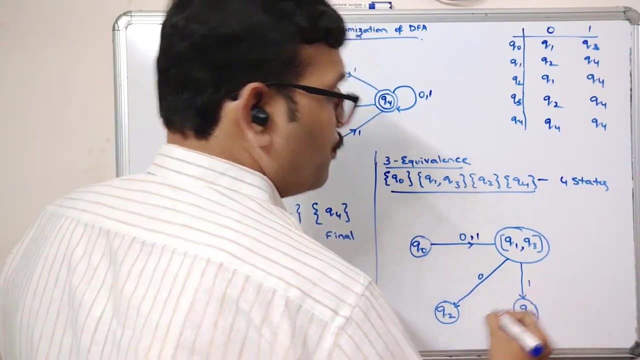 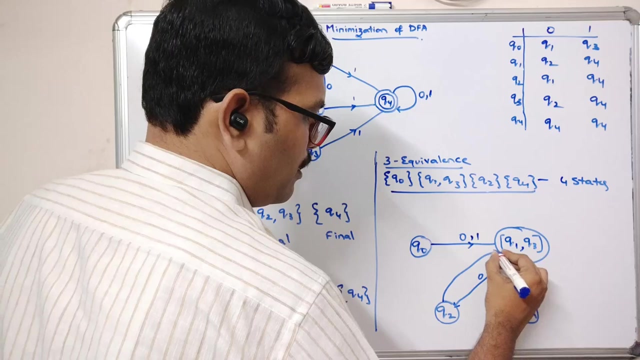 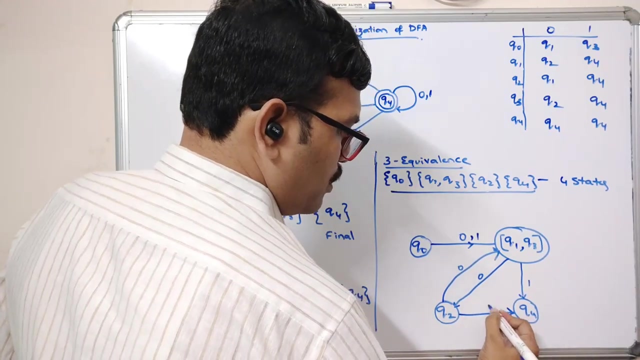 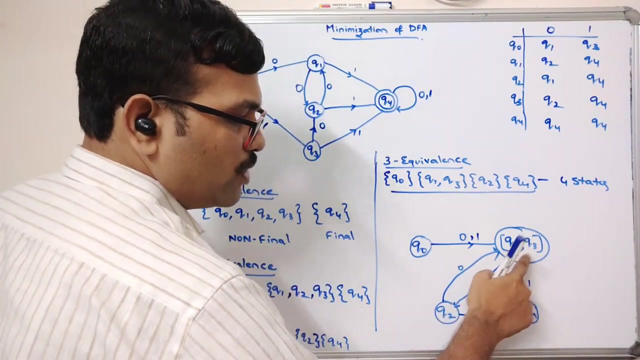 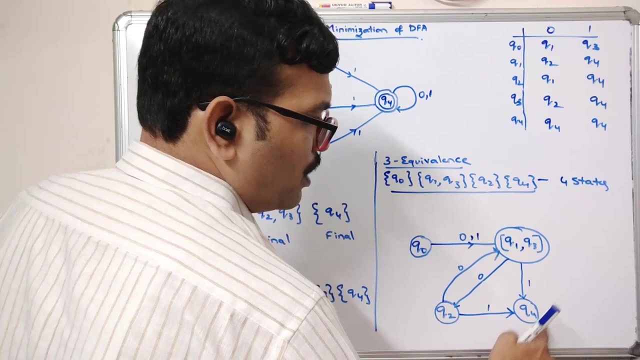 okay, and Q1 on 0 Q2. Q1 on 0 Q2, so Q1 on 0, it moves to Q2. next, Q1 on 1, it moves to Q4. Q1 on 0, 1, it moves to q4. q2 on 0 q1. q2 on 0 q1, so again 0. and q2 on 1 q4. q2 on 1, it is q4. q3 on 0 q2. q3 on 0 q2. so here you can see q3 on 0 q2. already there is a transition: q3 on 1 q4, q3 on 1 q4. 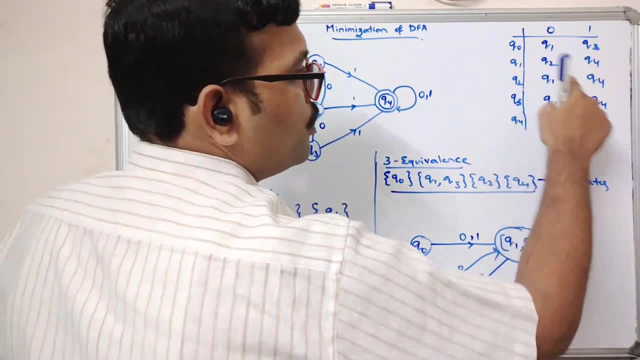 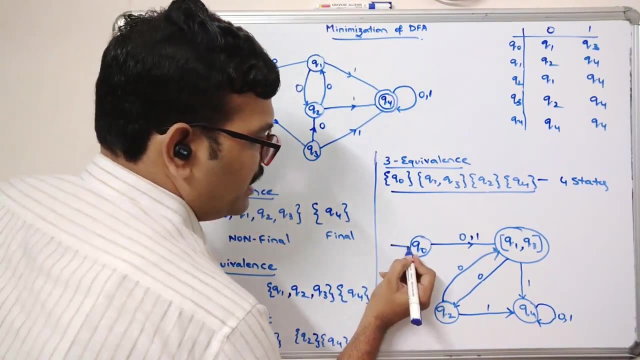 again. already there is a transition and q4 on 0 and 1. it remains in the same state. so this is the 0 and 1, so this will be the initial state. so here also, q0 is the initial state and q4 is the final. 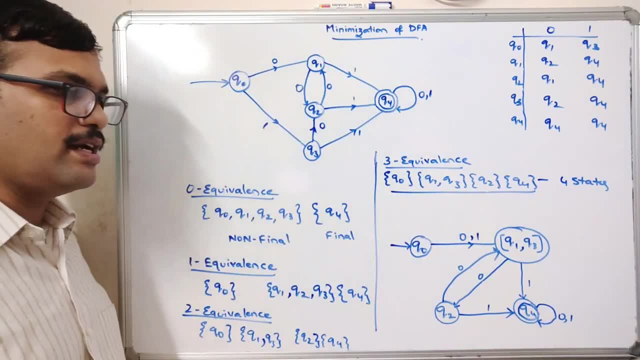 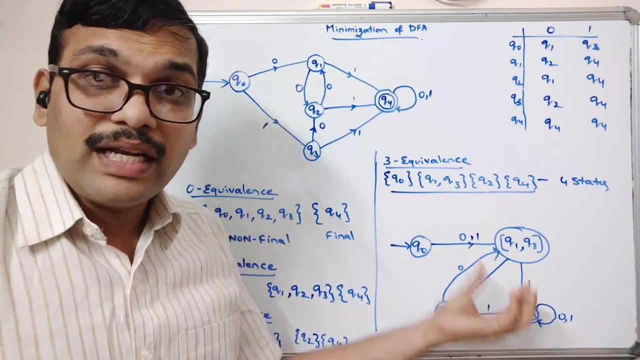 state and here also the q4 will remain the same as a final state. so we have, we are minimizing the given dfa to the another dfa, with a limited number of states, with a minimum number of states, right, and here you can observe the whether, whether, 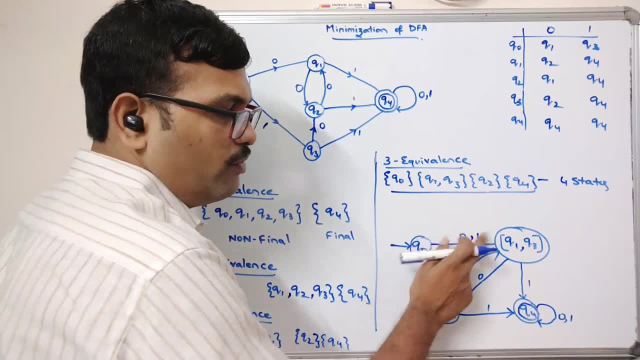 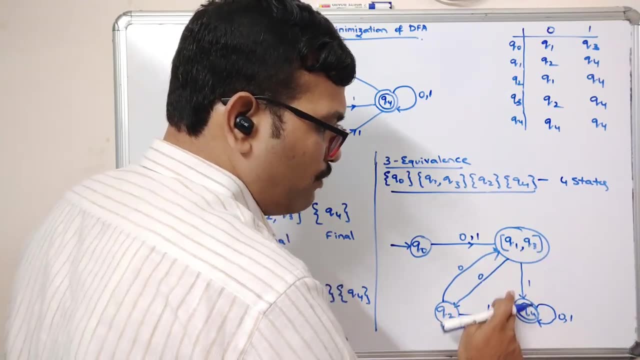 it is a complete dfa or not. so for q0, there is a transition for 0 and 1. yes, q2. for q2 there is a transition for 0 and 1 and q1. q3 is having a transition for 0 and 1. q4 is having a transition. 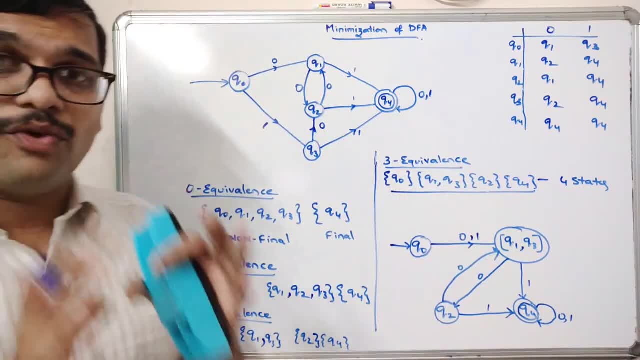 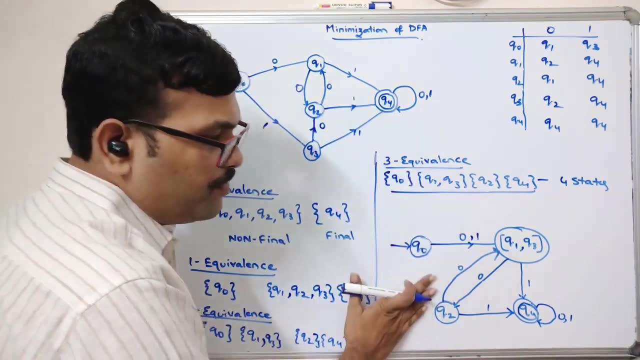 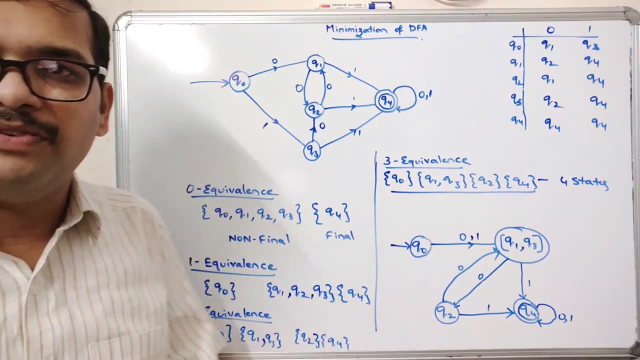 for 0 and 1. yes, so for every state there is a transition over every input symbol. so this is a complete dfa and we are minimizing this dfa to this dfa. that means we are reducing the five states to four states. so, simply by finding the equivalence between: 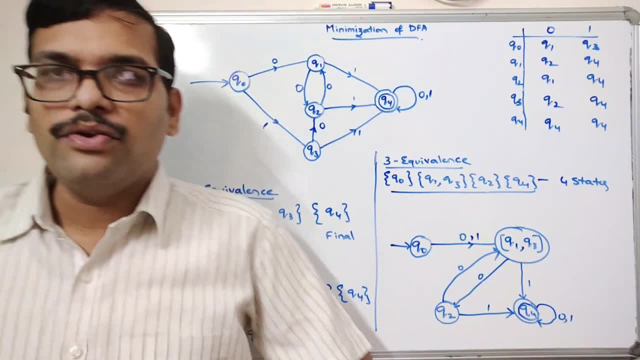 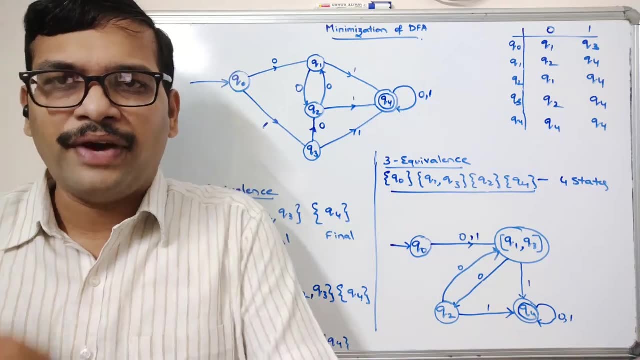 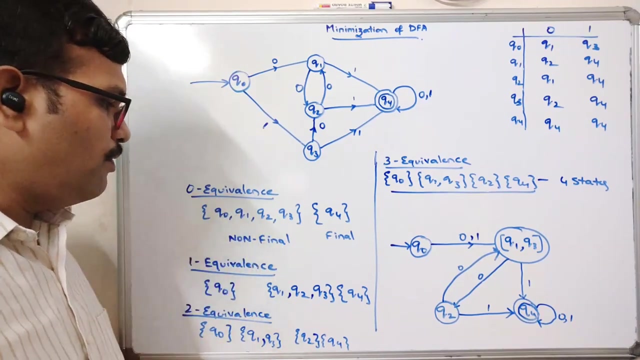 the states. so once again, i am repeating. so first we need to find out the zero equivalence, which is having a two sets- one set with the non-final states and another set with the final states- and from that we need to divide the complete states by finding the equivalences right. so for 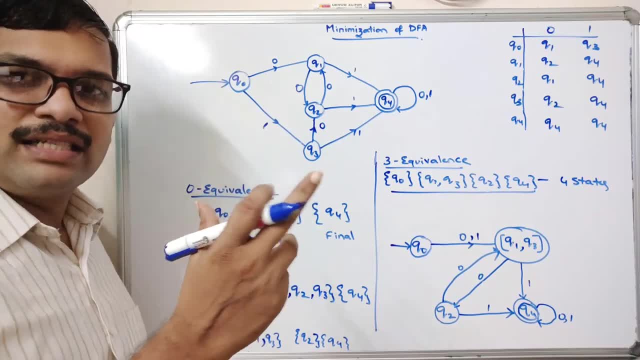 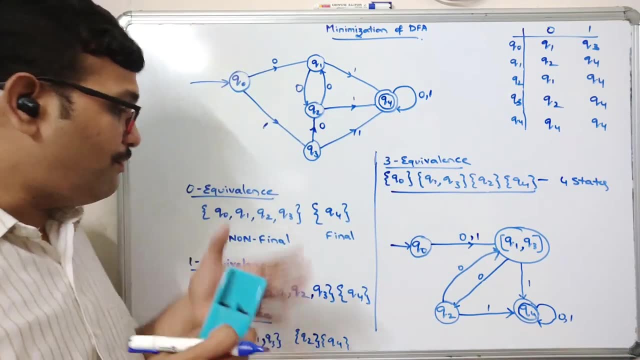 every state with the input symbols. we need to find the resultant state, whether they fall in the same set or not. if they fall in the same set, automatically the states are equal. and if they fall in different sets, automatically the states are not equal. so we have we have to divide in this one equivalence. 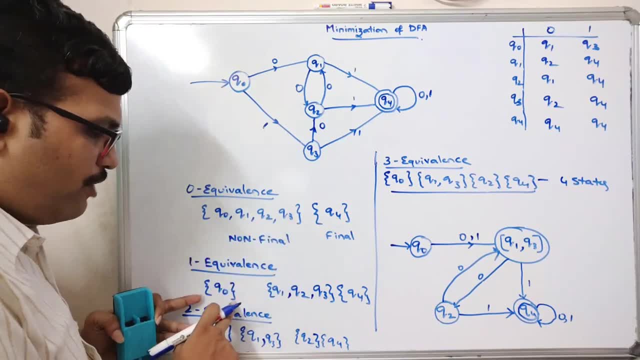 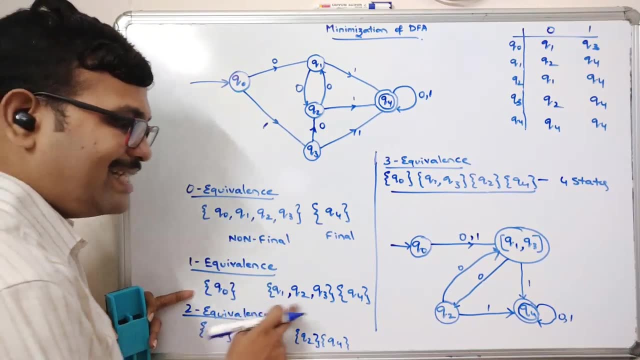 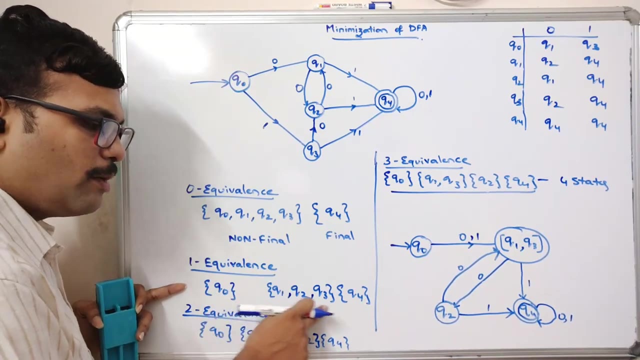 q0 is completely different with q1, q2, q3. so we have divided q0 with the q1, q2, q3 and q4. so here, after zero equivalence, we are getting the one equivalence with the three sets and from these three sets again you can find the three states with one set. we need to find the equivalence. 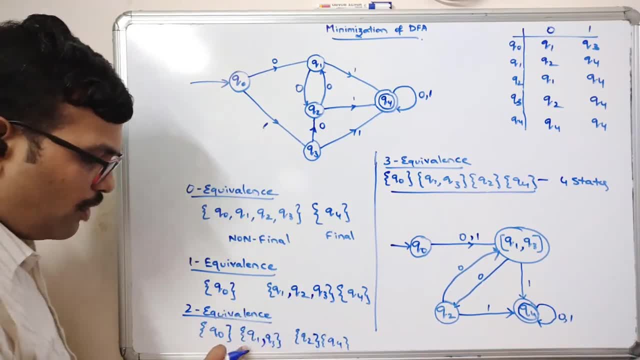 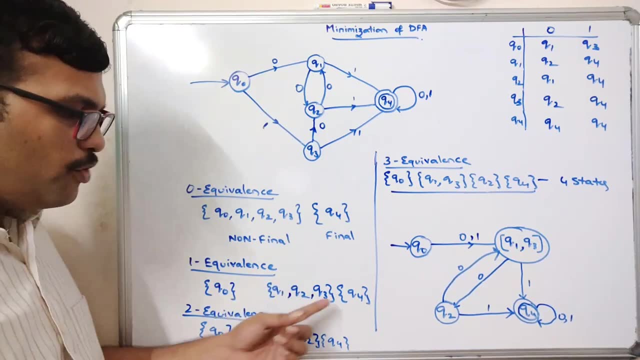 among these three states, q1 with q2, q3, so that we have: we got that q1 and q3 are equal and they both are not equal to q2. you can also compare q3 with q2, because here we are having some q1 and 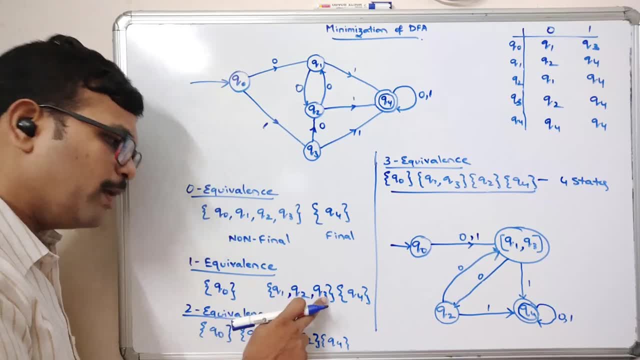 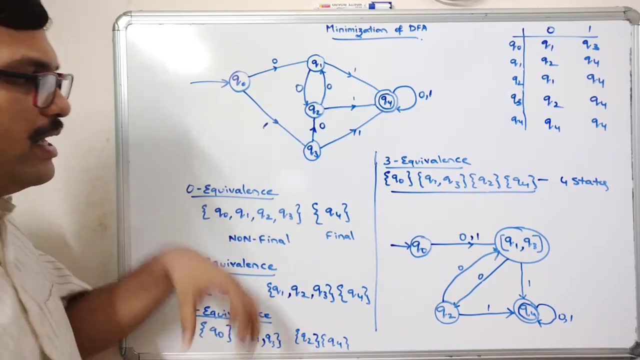 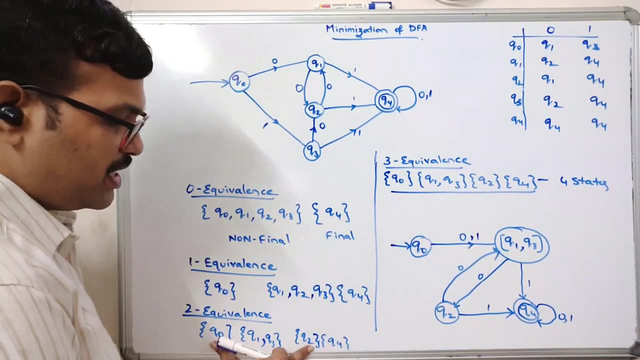 q3 are equal, so q1 and q2 are different. automatically q3 and q2 will also be different, right? so like this, we have to repeat the same process by finding the equivalences until you get last two equivalences as the same states. okay, so here you can observe: q0, q1, q3, q2, q4- four states: 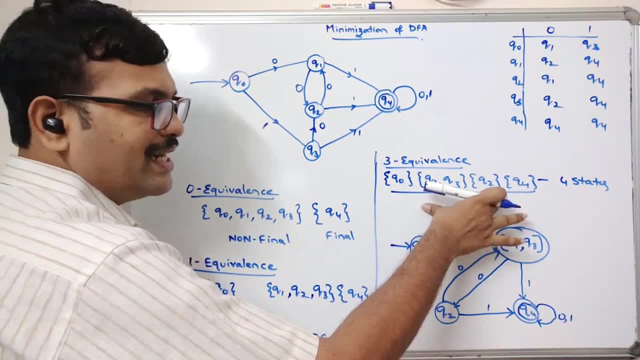 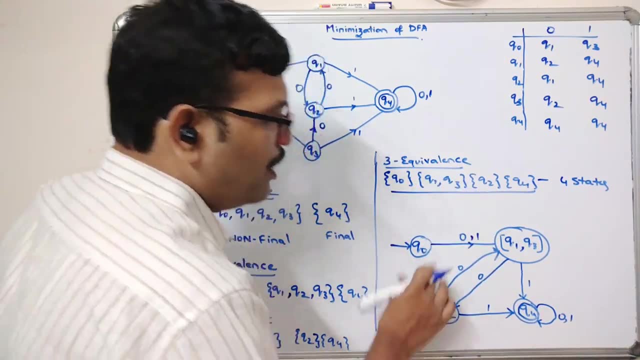 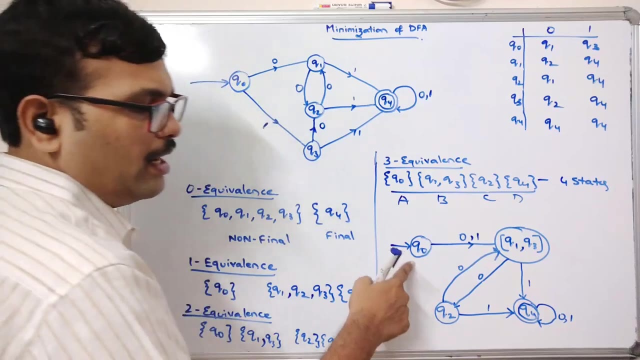 are there, four sets are there. and third equivalence: also the four sets with the same states. so that's why we have to stop at third equivalence and just draw the dfa with a given following states: so you can also rename this as a, b, c and d, and you can rename instead of using q0, you can use a, a instead. 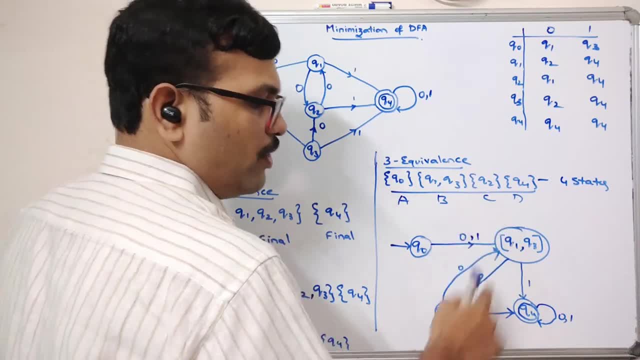 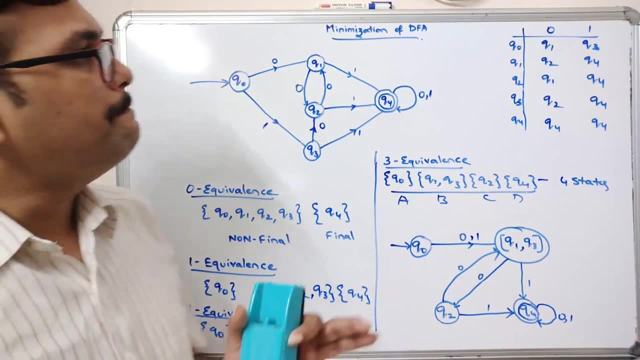 of using q1, q3, you can use a b instead of q2, you can use a c and instead of q4, you can use a d. right, so this is the procedure to follow, the i mean to find out the minimization of dfa right, and. 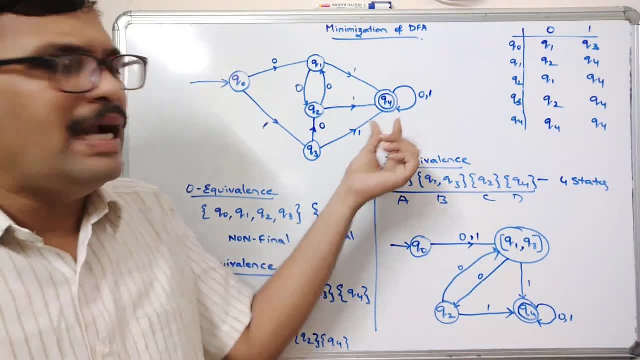 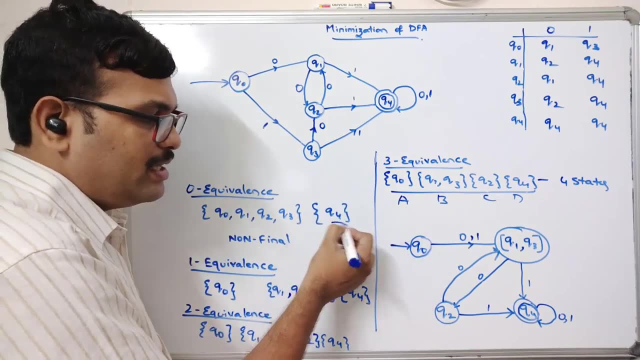 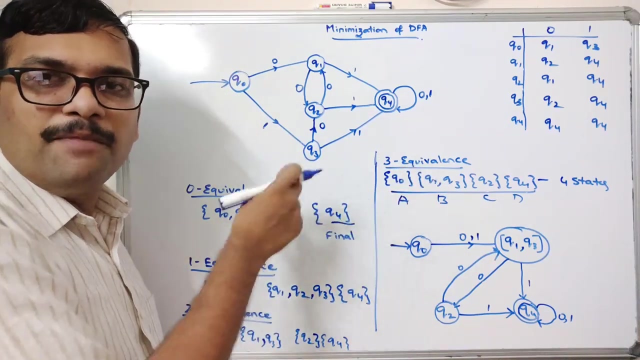 if in some dfa we are having a multiple final states, we have will be having a multiple final states, so here also, then in such cases we will get this set with a multiple final states and here also we need to compare each and every state of this final states. we have to follow the same. 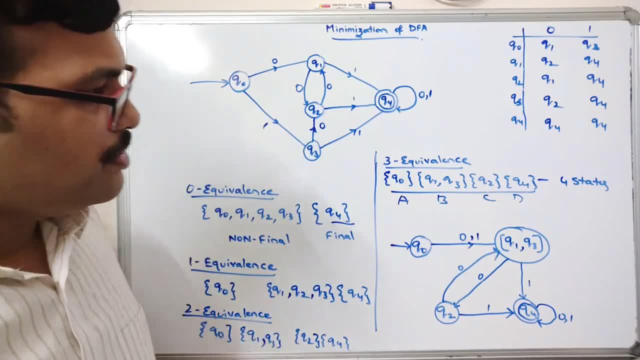 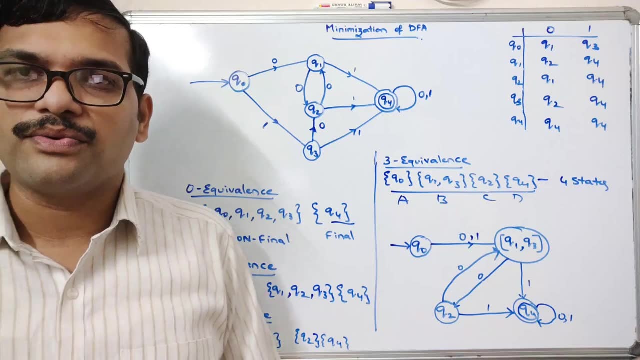 procedure right, so hope you understood this one. if you are having any doubts regarding this procedure, feel free to post your doubts in the comment section. i definitely will try to clarify all your doubts and if you really enjoyed my session, like my session, share my session with your friends. 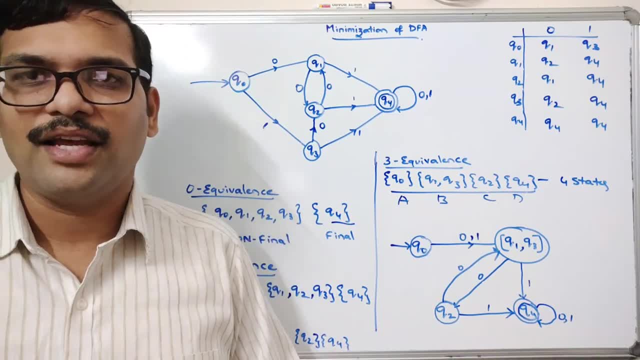 and don't forget to subscribe to our channel. thanks for watching. thank you very much. 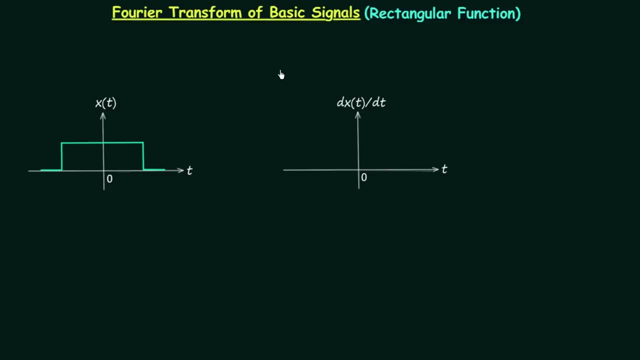 In this lecture we will calculate the Fourier transform of rectangular function And for this we will consider the general case. So the time domain signal xt is equal to a rect t over tau And we will calculate the Fourier transform of the rectangular function, Let's say the Fourier. 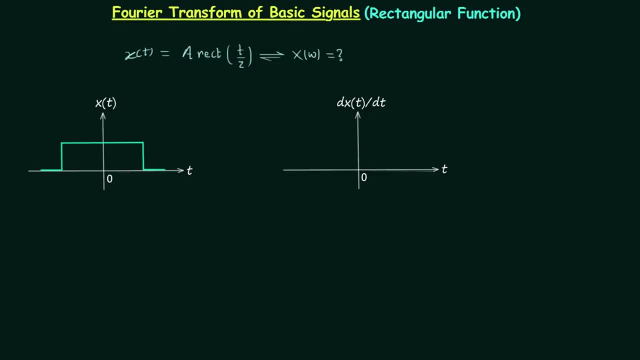 transform is equal to x, omega, And we know, in this representation, this a here is the amplitude of the rectangular function And this tau, here is the duration in which the rectangular function is having the value equal to a. So if this is the waveform of this rectangular function, then this: 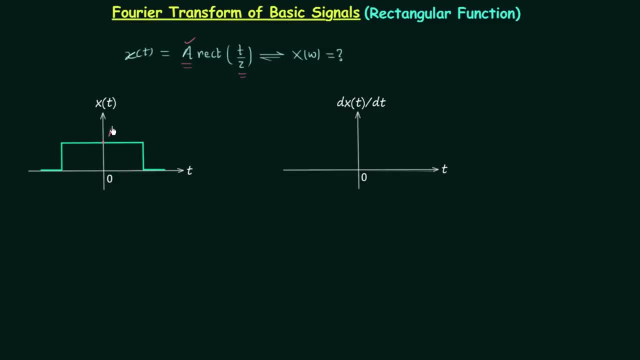 value of signal xt is equal to a, because this is the amplitude of the rectangular function And this is the amplitude of the rectangular function. And this is the amplitude of the rectangular function. And this duration of time is equal to tau, because in this duration the signal